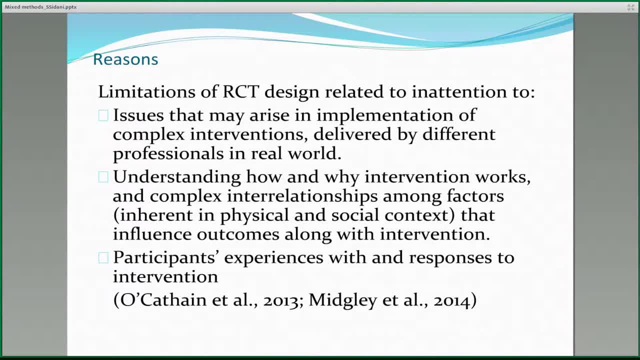 about them, but the most commonly mentioned limitations of the RCT that prompt researchers to use qualitative methods. Qualitative methods are one issues that may arise in the implementation of an intervention, but specifically complex interventions. By complex intervention I mean those that have 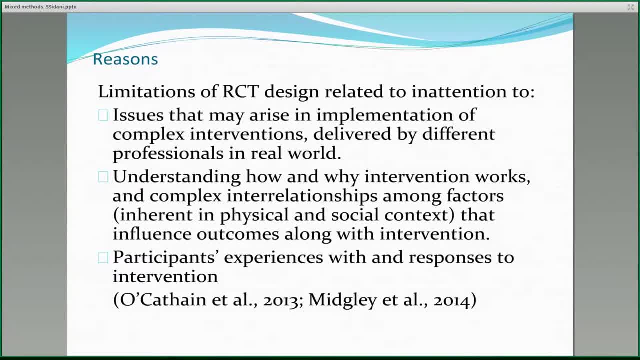 multiple components comprising them, And issues about implementation may arise when the complex intervention, or any intervention as a matter of fact, is delivered by different professionals in the real world. There has been also the concerns or critique of the RCT. is that it does not help The RCT. 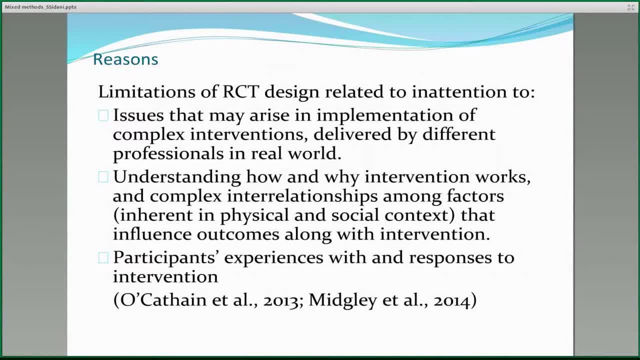 design does not usually help understand how and why interventions work and the complex interrelationship among factors that are present in the context in which the intervention is being delivered and or evaluated, that influence outcomes And we. there is enough evidence now showing that there are a lot of factors in this context. 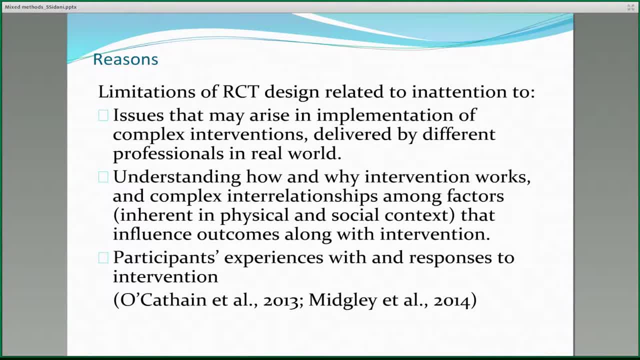 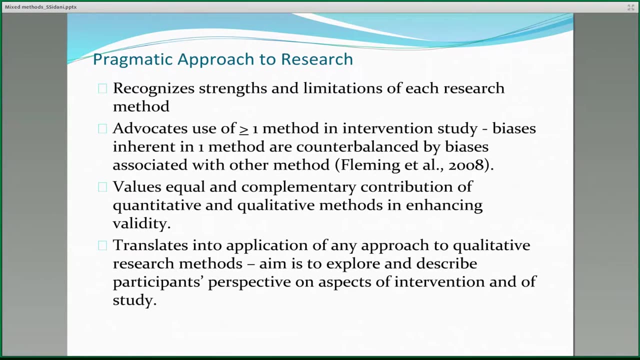 that could contribute to outcomes of an intervention and therefore should be accounted for when evaluating an intervention. The RCT also has limited attention to participants' experiences with and responses to the intervention, So these limitations led to the use of qualitative research methods within the RCT. 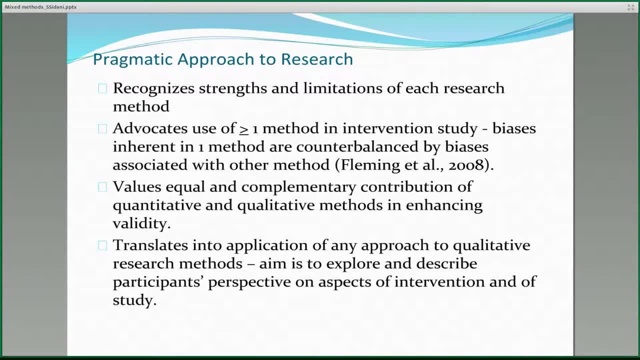 And I know that there are researchers, especially in nursing or some other health professions, but particularly in nursing, that have issues using both quantitative and qualitative methods within one study. This is where the approach here is a pragmatic approach that is used to help, if you want to call it. 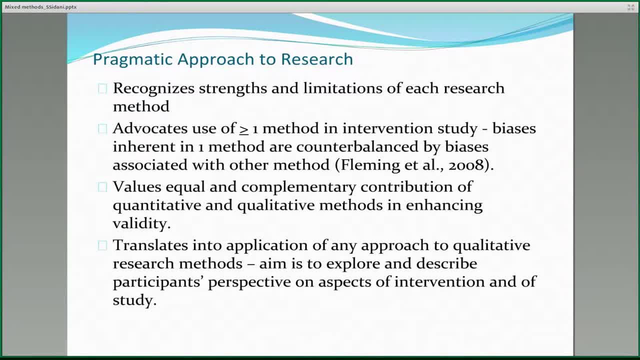 justify the use. So the RCT has the ability to use the use of two types of methods or approaches to research into one particular study: evaluating the intervention, of evaluating interventions. So this is called the pragmatic approach to research. It recognizes that each method has strengths and limitations. 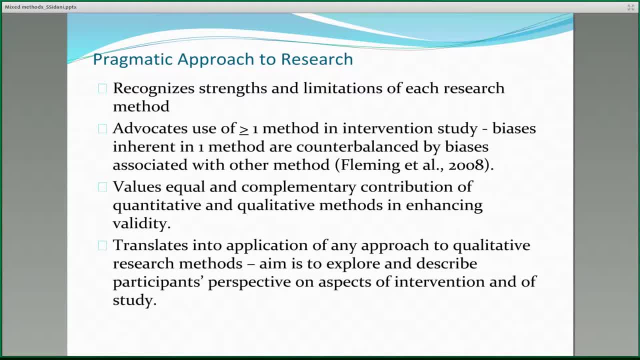 And therefore, because each one has a strength and each of the qualitative has and the quantitative has strength and limitation. and therefore, because each one has a strength and each of the qualitative has and the quantitative has strength and limitation. and therefore, because each one has a strength and limitation. therefore, using the two or more than one method, 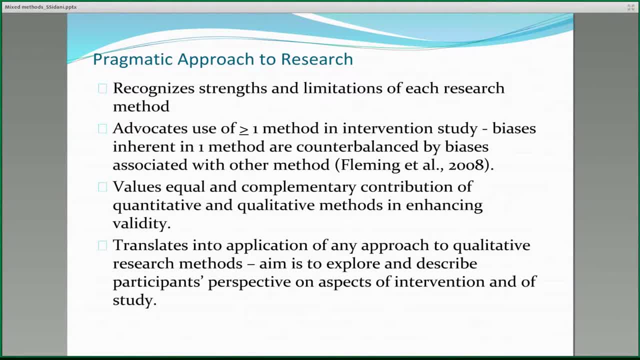 in an intervention study is important as a mean to minimize the potential biases inherent in one method, So that if you are using qualitative that has strengths and limitation and or biases inherent in it, and quantitative that have similar biases inherent in them, by using the two, you know you will counterbalance these. 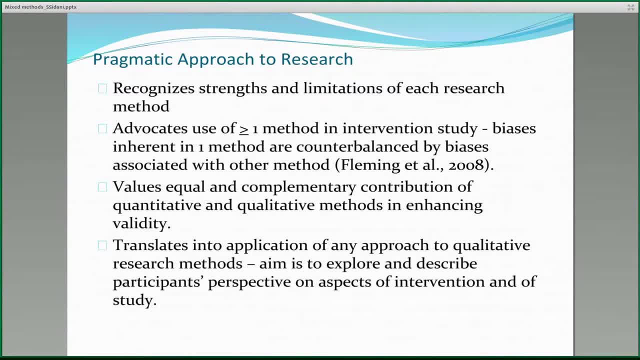 the two you know you will counterbalance these. the two you know you will counterbalance these biases. So it's a very pragmatic approach to using different methods within a particular study. The pragmatic approach also values the equal and complementary contribution of each method. 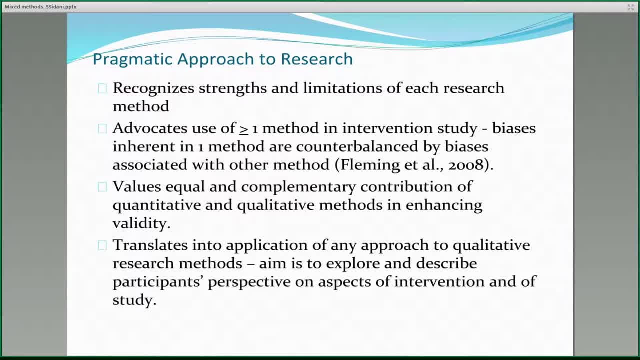 within a particular study, because each one will contribute something different, complement each other, corroborate the findings from each other, which leads to improvement in the validity of the conclusion. Lastly, the pragmatic approach translates into the application of any type of qualitative research methods into the RCT. 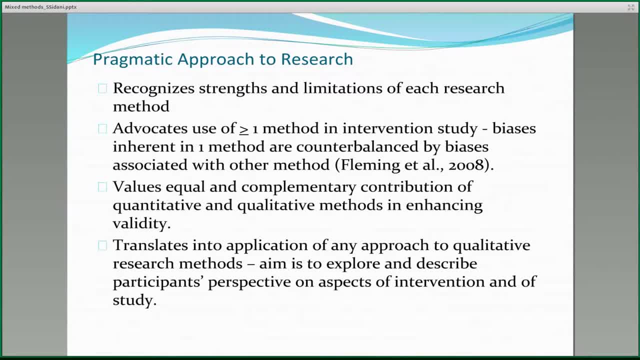 And I'm saying any type or any approach to qualitative methods, meaning that you know, the literature discussing the use of qualitative or mixed method in an RCT does not really specify whether you need to use a phenomenology or grounded theory or whatever. 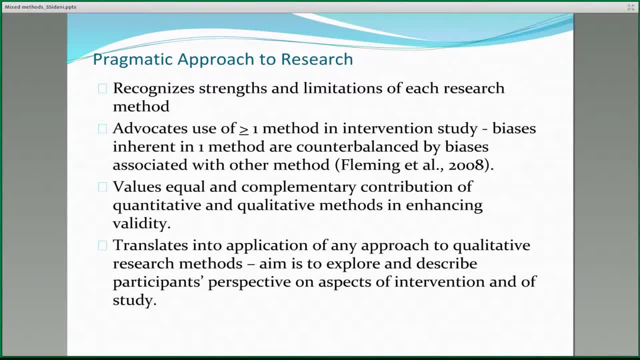 So you can use a qualitative method regardless of the theoretical or philosophical assumptions underlying it, because the aim here, within this pragmatic approach, is to explore and describe the participant's perspective on different aspects of the intervention and or different aspects of the study or the trial. 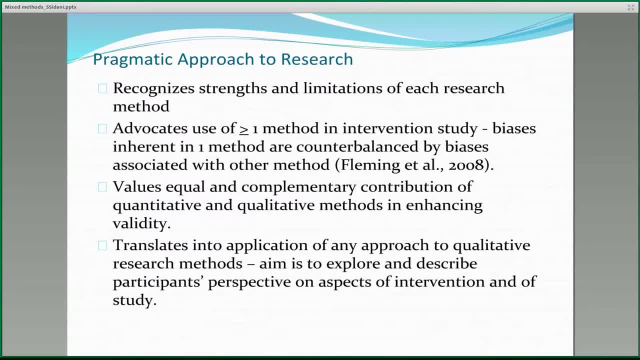 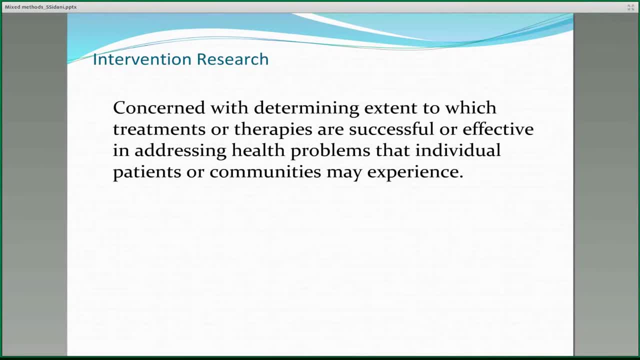 Thank you, Thank you, Thank you. So these were the foundational points that I wanted to clarify before we move into the use of mixed methods in intervention evaluation research, which is concerned with determining the extent to which an intervention or a treatment or a therapy is successful and effective. 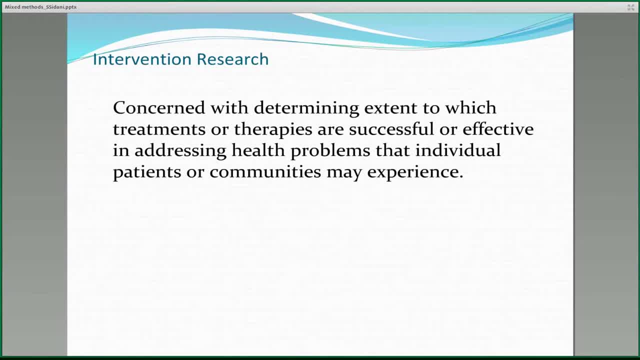 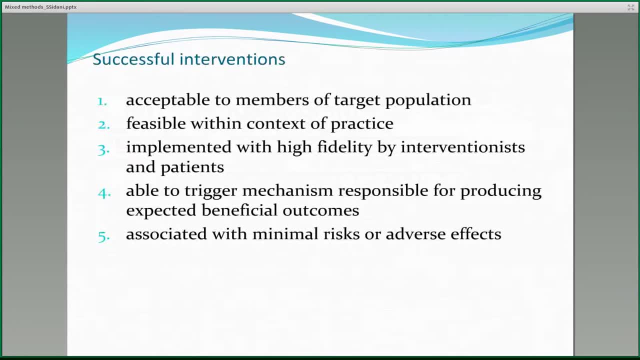 in addressing a health problem that may be experienced by individuals, whoever the target population is- It could be a patient, or the patient or the community itself- And usually a successful intervention, or an intervention is considered successful if it is acceptable to members of the target population. 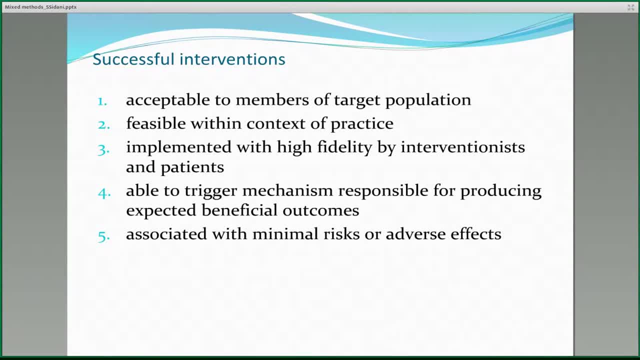 if it is feasible within the context of practice, if it's implemented with high fidelity by the interventionist as well as by patients, and able to trigger the mechanisms responsible for producing the expected benefits Or beneficial outcomes or changes in the outcomes, And the intervention should be associated. 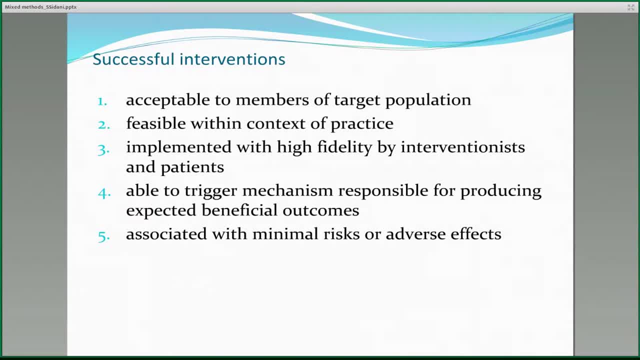 with minimal risk or effects. It's only when an intervention meets all these five criteria, if you want to call them, that an intervention is considered successful and therefore ready to be disseminated and incorporated in the day-to-day practice. So to demonstrate the successfulness of this, 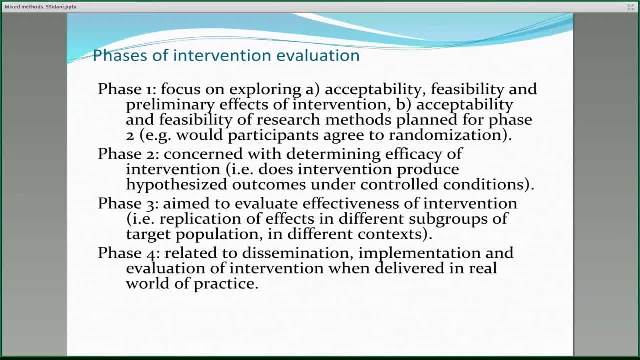 and the success of these interventions. the interventions are usually evaluated in four phases. The phase one is more of a pilot study. We're exploring the feasibility, acceptability, as well as the preliminary effects of the intervention, And by preliminary effect I mean here. 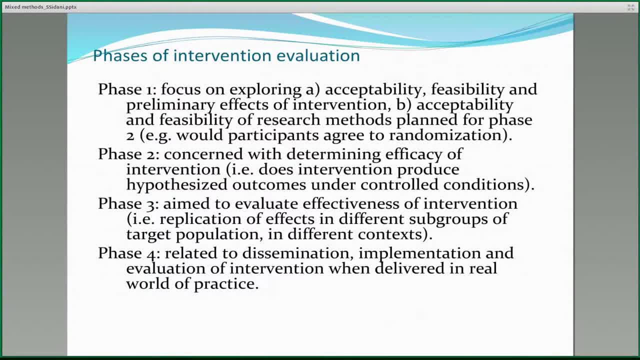 that the intervention is able to produce or to induce some of the changes expected in the outcomes. And in a pilot study, also a phase one trial, the focus is also on examining whether or not the research methods are acceptable and feasible, In particular, issues around recruitment retention. 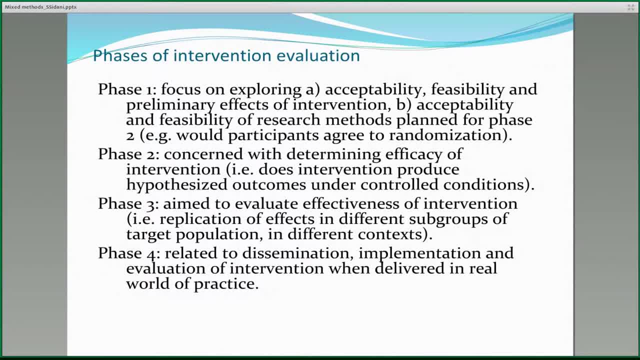 and whether or not participants would agree to randomization, And I'm highlighting randomization because a lot of research now showing that participants do not like randomization. Phase two trial is concerned with determining the efficacy of an intervention, meaning that it does produce the outcomes. 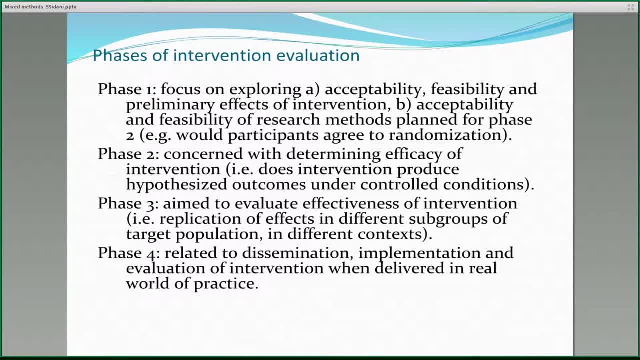 under the controlled conditions, Whereas phase three, it evaluates the effectiveness of the intervention, meaning whether or not the changes and the beneficial changes in the outcomes are replicated in different contexts, And by context I mean here different populations or subgroups within a population. 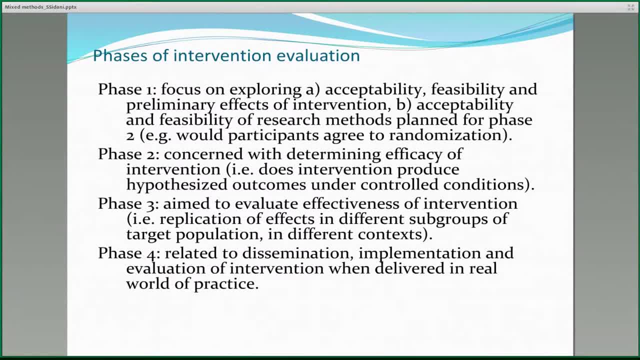 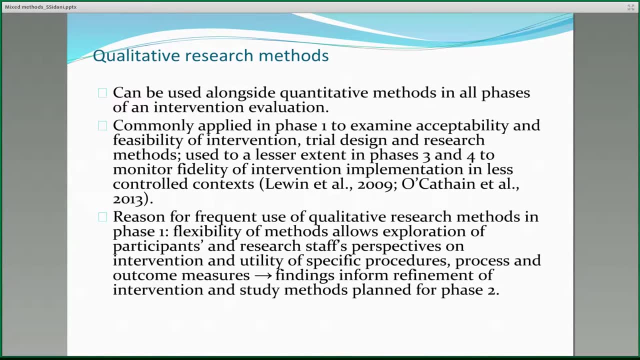 different settings. And the last phase, or phase four, is related to the dissemination and implementation of the intervention when delivered in the real world. Qualitative research can be used along any of these phases for evaluating intervention. However, they have been most commonly. 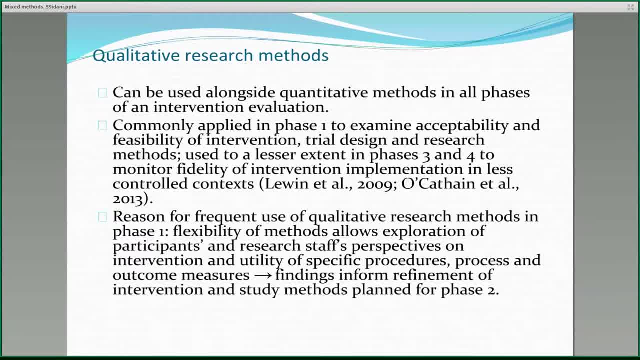 based on my read of the literature, they have been most commonly used in the field of clinical research. Now I want to talk a little bit about the different processes applied or used in the phase one pilot studies to examine the acceptability as well as the feasibility. 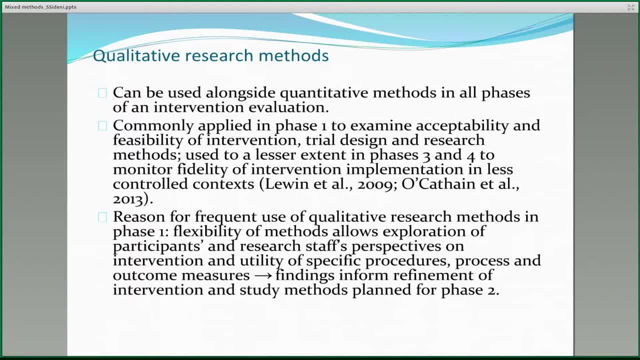 of the intervention, acceptability and feasibility of the trial, design and research methods. They have been used to a lesser extent in the phase three and phase four And, if used in these phase three and phase four, looking at the fidelity, looking at the efficacy or effectiveness. 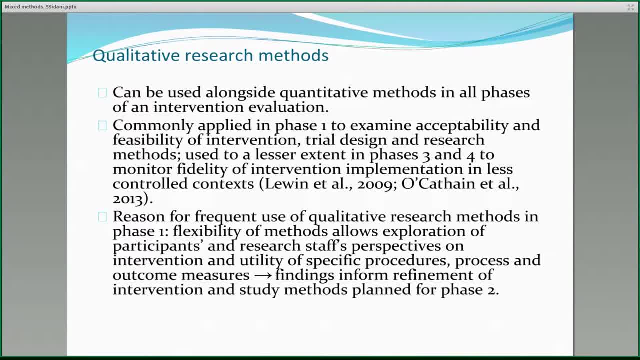 of an intervention. usually, qualitative methods have been used primarily to monitor the fidelity with which an intervention is being implemented. We do not know the exact reason for why qualitative research methods are used more in phase one, But what has been suggested in the literature is that with these qualitative research methods, 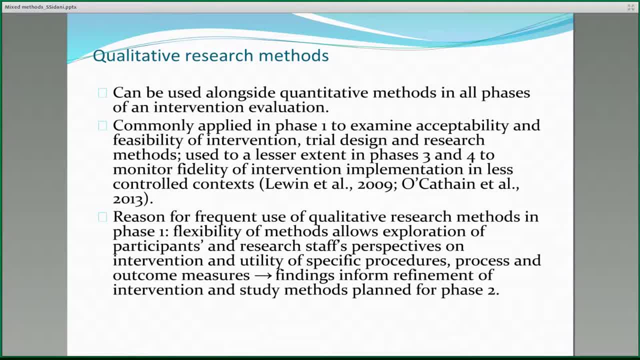 there's more flexibility in what can be done with them, How to implement them and how to use them, And they can be used also to collect data on these participants and the research staff perspectives on the intervention By using the term perspective they're. 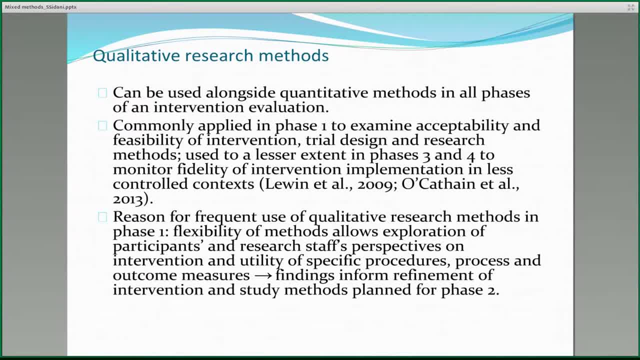 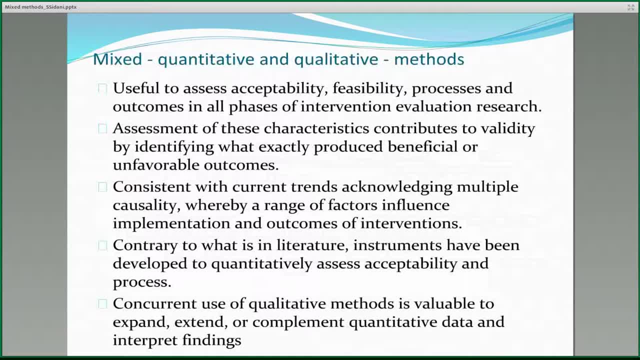 keeping it kind of wide open in terms of what a researcher would like to examine, in particular about this perspective, What I would propose today, Thank you. So I think what I would say is that a mixed method, quantitative and qualitative methods, 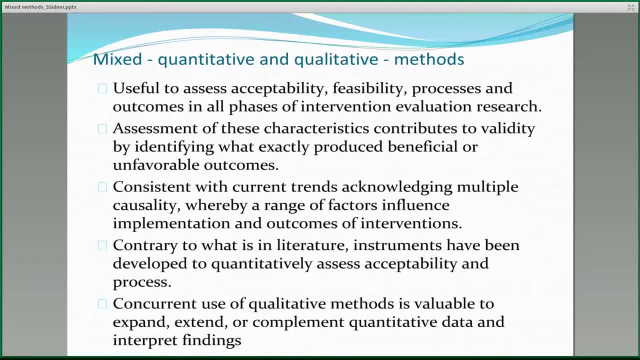 could be useful to assess the acceptability, feasibility processes as well as outcomes of an intervention in all phases, And not only phase one or phase two, but all of these aspects of an intervention could be evaluated in efficacy as well as effectiveness trial. 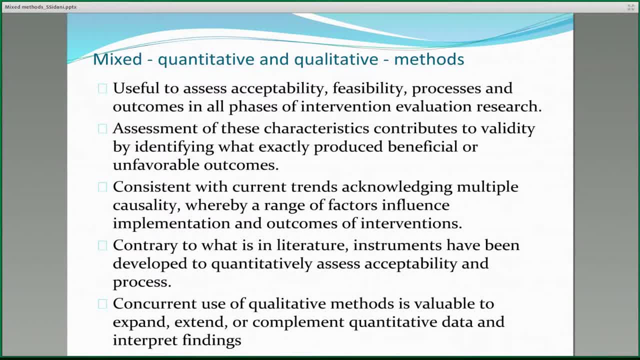 And they are not necessarily only focused pilot studies. The assessment of these characteristics contribute to the validity of the study's conclusion, as we will discuss throughout the rest of this webinar, And the use of quantitative and qualitative methods to assess acceptability, feasibility, processes and outcomes is consistent with current trends that acknowledge multiple causality. 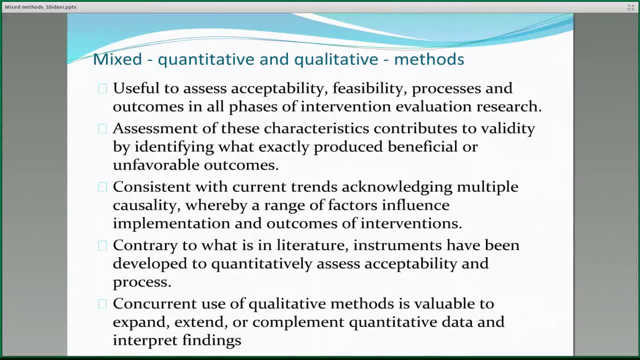 By multiple causality I mean that there's now more and more recognition that there are other factors besides the intervention that could influence or contribute to the achievement of the outcomes, and therefore we need to assess all of those factors if we would like to reach various outcomes. 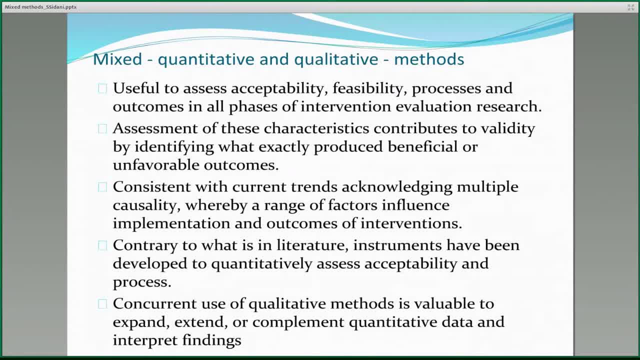 So I think that's really valid conclusions about what exactly is contributing to the observed outcomes, And this becomes important because you will see in some of the examples, there may be aspects of the intervention delivery itself that leads to improvement in the outcomes, rather than the intervention active ingredients. 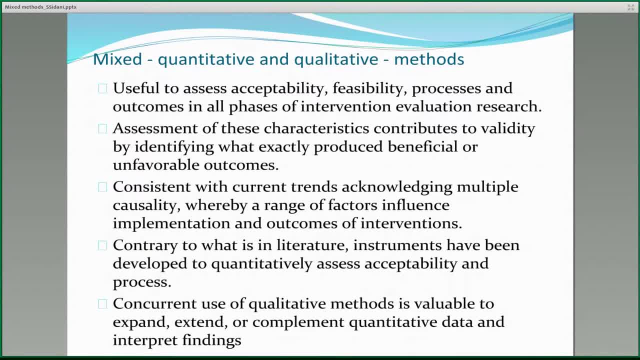 All I wanted to say in these last two points within the slide is that most of the liver literature articles that you would read about using qualitative methods within an RCT do say that qualitative are important and useful, which I would acknowledge to examine acceptability. 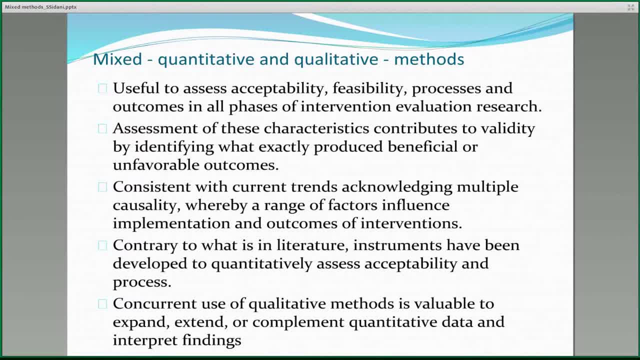 and you know, or process of intervention implementation, But I just wanted to let you know that there has been enough now scales that have been developed to assess acceptability and feasibility. Thank you, Thank you, And just in terms of the implementation of an intervention, just claiming that you want. 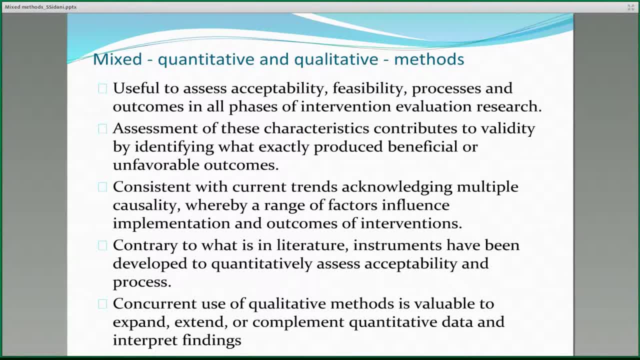 to use qualitative to assess these two aspects is not, in my opinion, a very strong argument for using qualitative, because there has been also quantitative measures of these two aspects of an intervention. This is why I call this a presentation using the mixed method. Thank you. 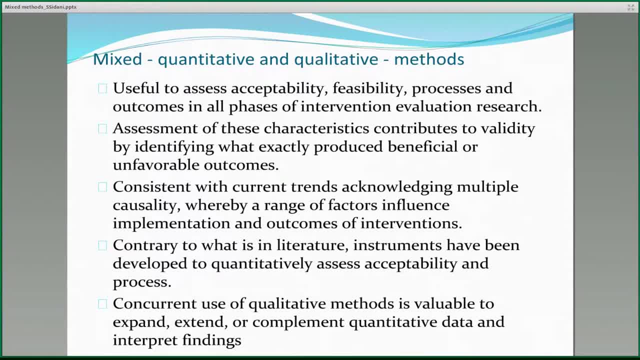 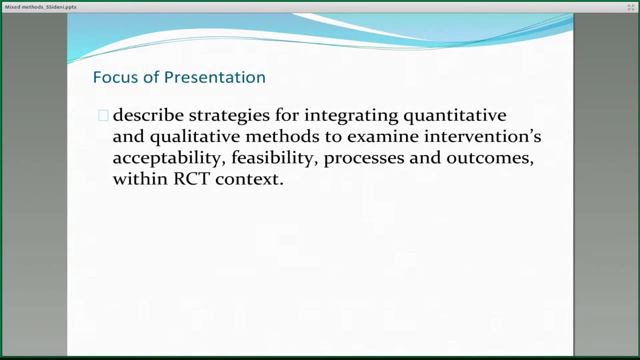 for evaluating an intervention, and the two, qualitative and quantitative methods, can be used concurrently and are valuable to expand, extend, complement each other and they are very helpful in the interpretation of findings. So the focus of this presentation is on how to integrate quantitative and qualitative. 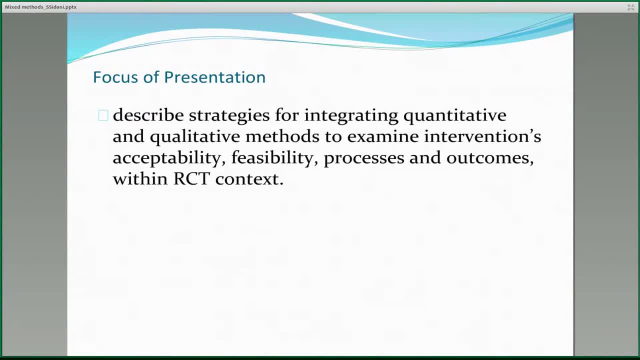 methods in examining the intervention acceptability, feasibility, processes and outcomes within the context of an RCT. I will not discuss the use of mixed methods for evaluating research designs and methods, because there's plenty of articles that discuss those, So I'm focusing only on the evaluation of an intervention. 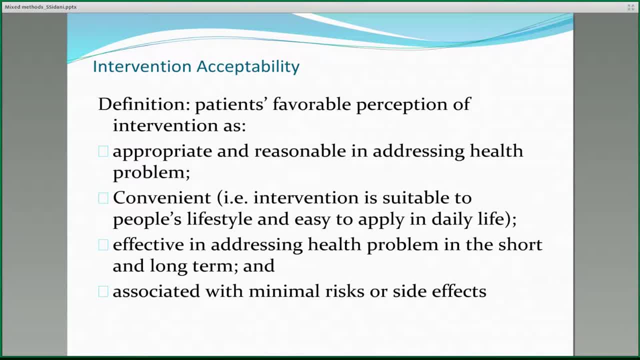 The first aspect of an intervention where the mixed quantitative and qualitative methods could be used within an RCT is to examine the acceptability of an intervention, and acceptability here refers to the patient's favorable perception of an intervention. What do we mean by favorable? 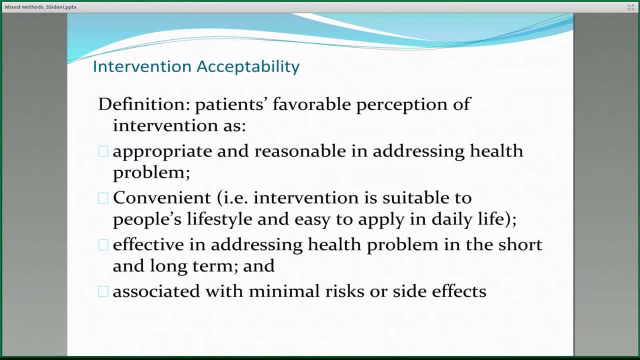 Meaning that the patient or participants would consider or view or weight or judge the intervention as appropriate and reasonable in addressing the health problem that they may be experiencing and for which they are seeking treatment. They would also consider the intervention as convenient and the convenience is becoming. 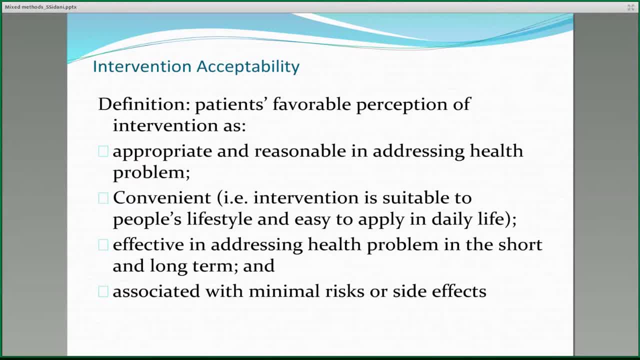 meaning that the intervention is suitable to their lifestyle and it's easy to apply in their day-to-day life, and this is becoming a very important attribute of an intervention. that influences a lot of participants' perception of an intervention. They also have to consider or perceive the treatment as potentially effective in addressing 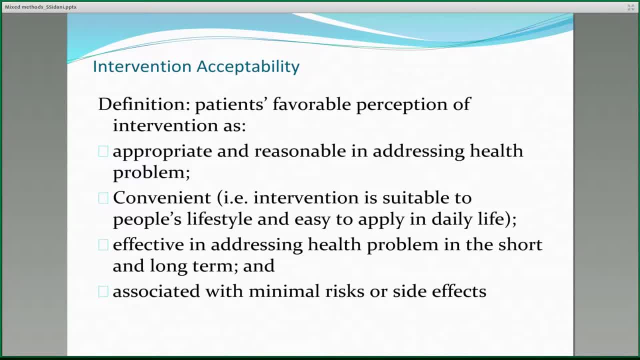 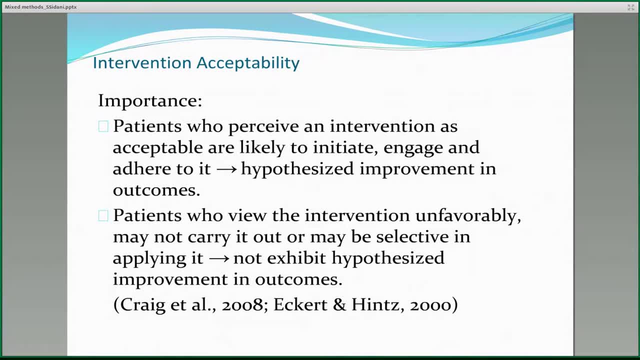 their problem in the short term and the long term, and it's associated with minimal risk or side effect. Why is it important to examine acceptability in any intervention evaluation study, Not only in the phase one or pilot studies, because there's not enough evidence to show. 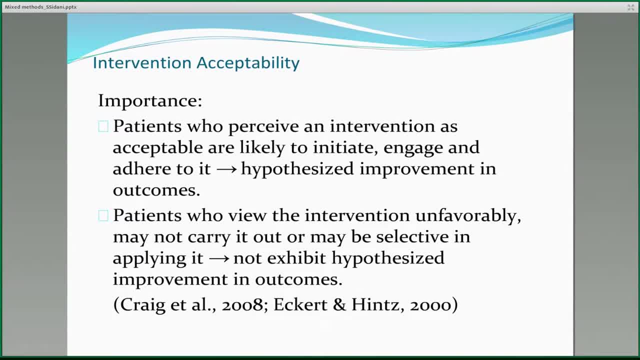 that patients or participants who perceive an intervention as acceptable are likely to initiate it, to engage in it and comply with it. And if they comply or adhere to this intervention, then at that point they will demonstrate the hypothesized improvement in the outcomes. In contrast, if patients view an intervention as unfavorablyunfavorably sorry and they 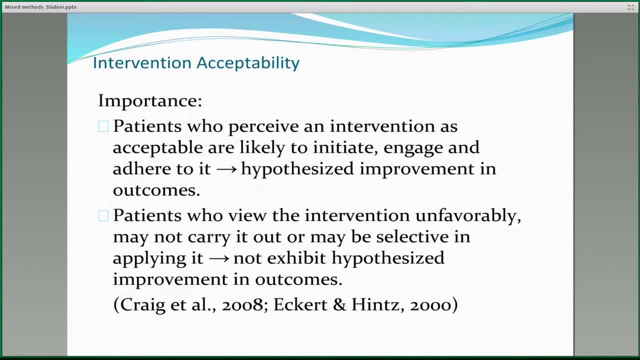 may not carry it out or they may be selective in what aspect of the intervention they may apply. So they may apply one component or another component, but not all of them. And if you know they are selective at applying some component but not all, then they may. 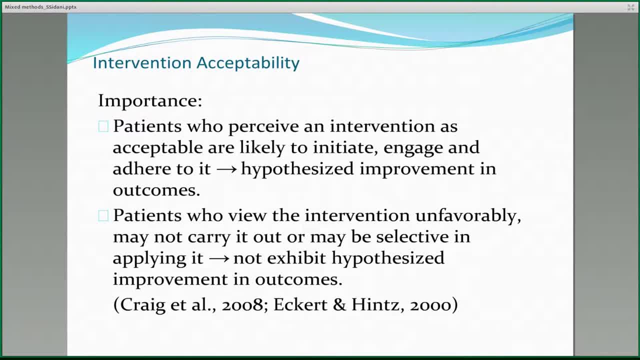 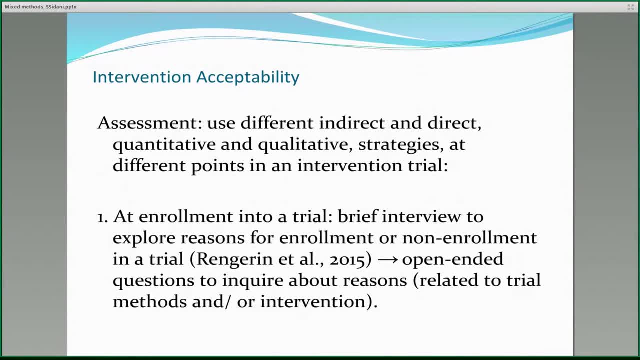 not benefit from this intervention. So how can we assess acceptability? Acceptability can be assessed, Okay, in different direct and indirect methods, quantitative and qualitative strategies, And the assessment of acceptability can be done at different points within an intervention trial. 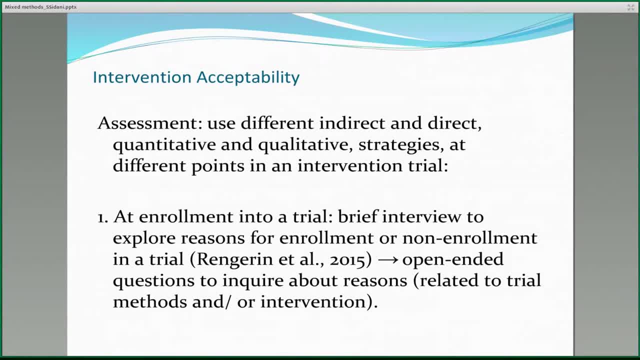 So at the trialat the enrollment in the trial, you can askyou can have a brief interview to explore reasons for enrollment in a trial or reasons for non-enrollment, as has been done by or suggested by. You can use open-ended questions where you can ask participants about the reasons for. 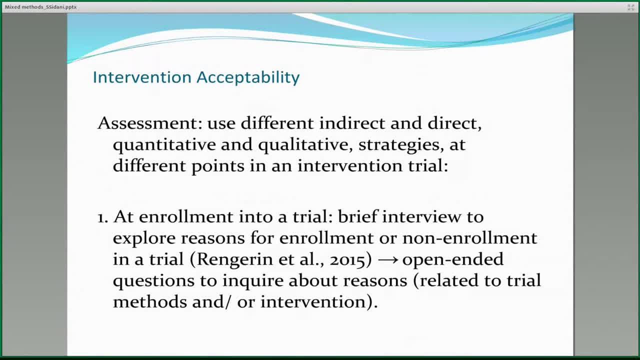 not participating and look for reasons that could potentially reflect their perception of an intervention such asor reflect their acceptability of the intervention. Example of terms that we have usedI'm sorry that we have heard that were indicative of possibleof possible unacceptable intervention are something like the treatment is demanding. 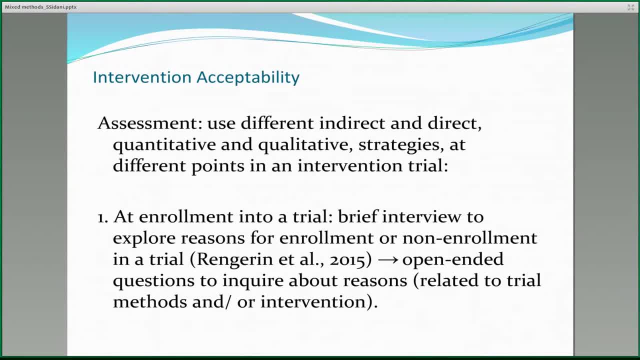 or I do not like the treatment, And I will consider these as indirect indicators of acceptability. I just want to remind myself, as well as everyone who's listening that tonow, with the changes in ethics requirements, towe need it to get the participants' consent in order to. 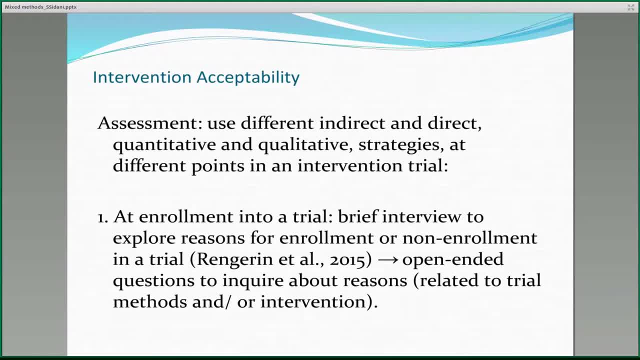 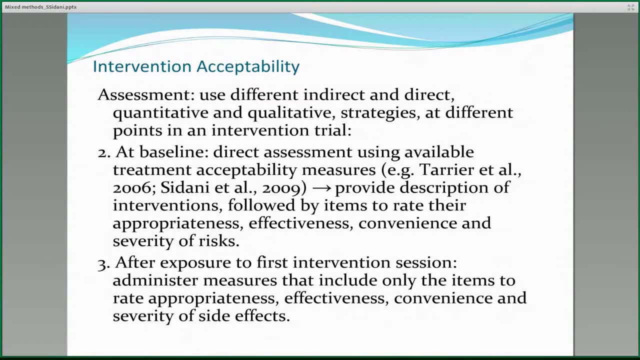 make this happen. Okay, Thank you. consent in order to conduct these brief interviews. Acceptability can be also assessed at baseline, after obtaining the consent and collecting pretest data. This can be done here directly using a direct assessment with measures that have been developed. 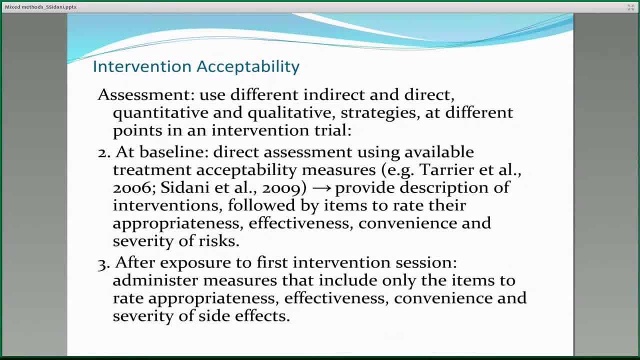 and validated to assess the acceptability of an intervention. An example of these measures are the ones developed by Terrier and my colleague and myself. These measures usually provide a brief description of the intervention and it is important at baseline to provide a brief description of the intervention so that participants would 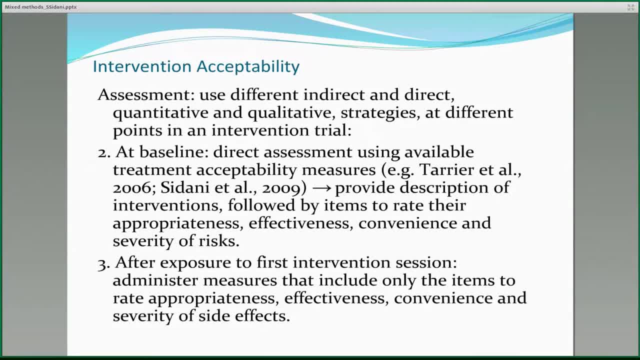 get a sense of what the intervention is all about, And the description is followed by items that would ask participants to rate each intervention under evaluation, And that may include the experimental intervention as well as the control or the comparison condition. You ask them to rate it at baseline, to rate each one in terms of its appropriateness in 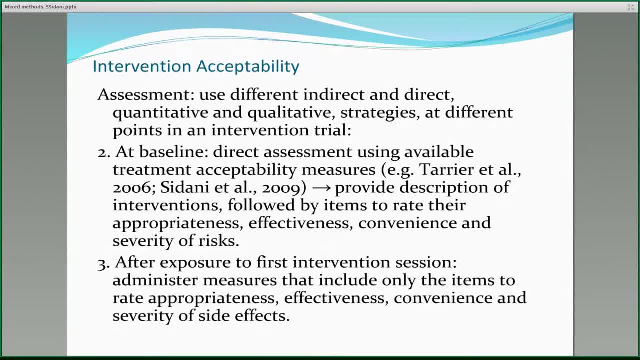 addressing the problem, its effectiveness, convenience and side effects, or what they're doing, Acceptability, can be also assessed after the exposure to the first intervention treatment, as has been done a lot in psychology, where they administer a questionnaire that they tend to call credibility of the intervention or of the therapy session. 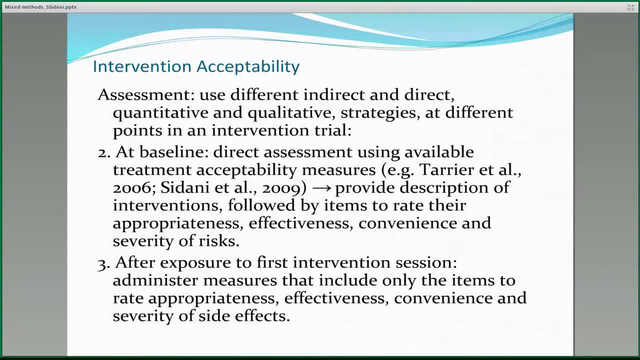 And at this point in time, because they have been exposed to the side effects of the intervention, some aspect of the intervention, you do not need to give them the description of the intervention, but ask them just to rate it using the items that assess appropriateness. 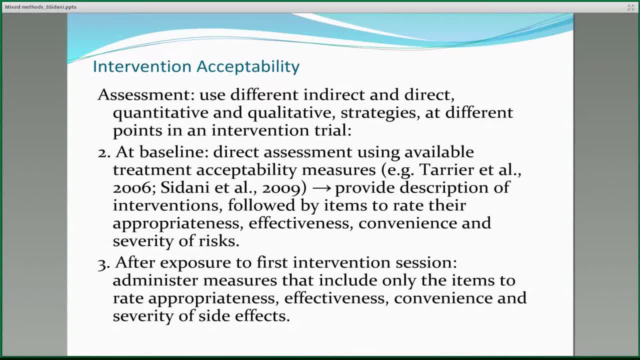 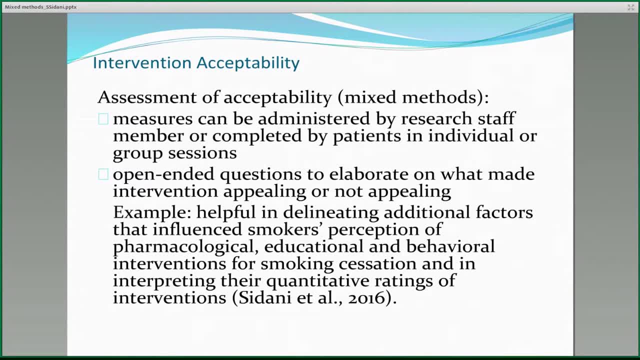 effectiveness, convenience and severity of the effect These acceptability measures could be used. they can be administered by the research staff or they can be completed by patients and individuals. They can be used in individual or group sessions, whichever is most convenient and appropriate. 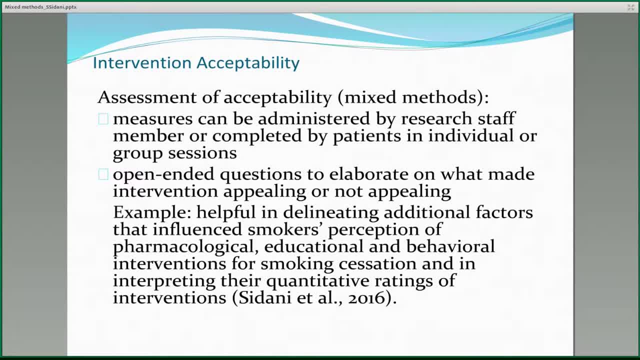 and feasible within your intervention evaluation studies. I have used these as measures to assess acceptability in a group format as well as individual format, where you know participants would read the information and complete the measures, And I follow them usually with open-ended questions. 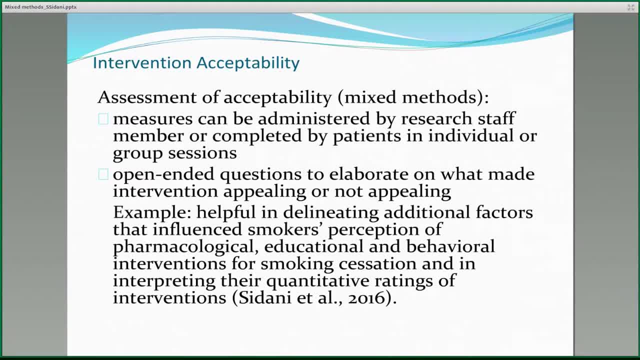 To asking them, asking the participants to elaborate on, you know, in their own words, what made this intervention appealing or not appealing to them. We found this intervention, you know, the use of the mixed methods where to assess acceptability, where people have to wait each intervention and then we ask them these open-ended questions. 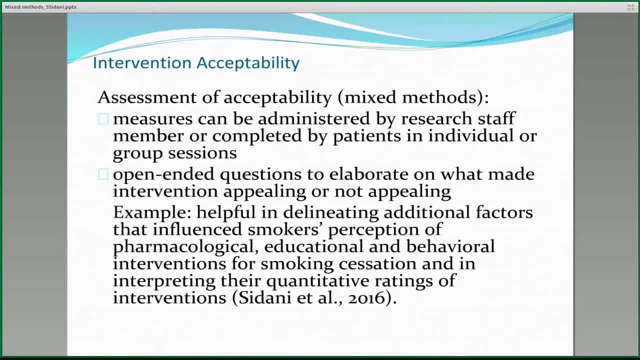 very useful in helping us identify additional factors that patients may or participants may not have. And participants do take into account when they are reading and determining which intervention is acceptable to them. And you know we do have the results of these mixed method approach of assessing acceptability. 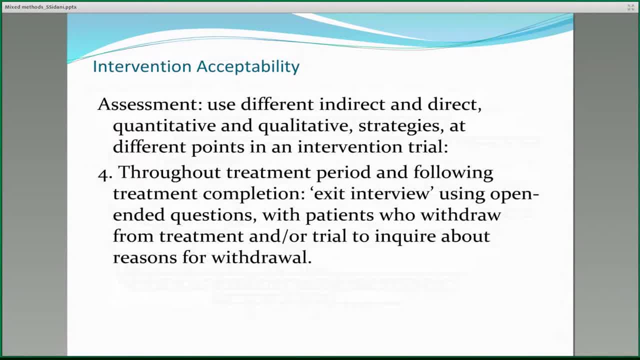 published in 2016.. Acceptability can be assessed throughout the treatment period If anyone is interested, but particularly at the and you use it throughout the treatment period if you have a complex intervention where each component is delivered- a different session, for instance- and you would like to examine or assess the acceptability of. 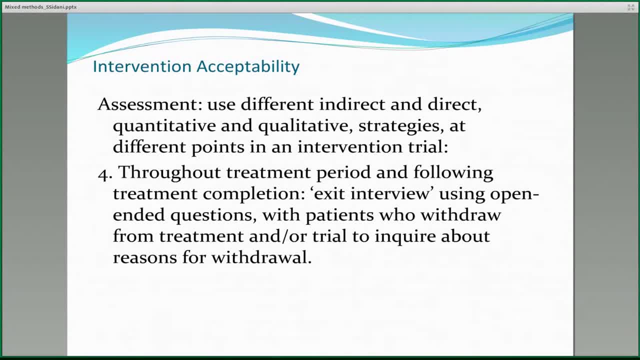 the different components. Or you can do it at the completion of the treatment, using some form of- again mixed method where you ask them also to complete the same measures or other measures- Okay, So you ask them to complete the same measures or items assessing acceptability and use, and. 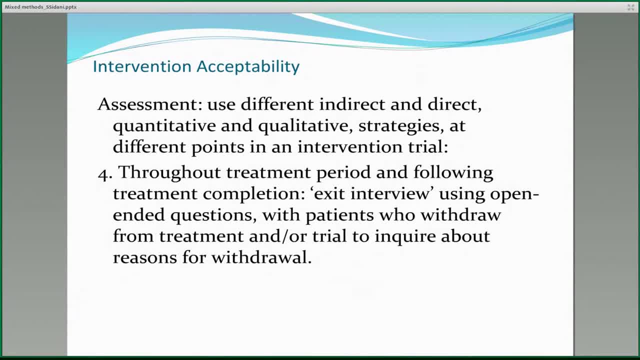 all. so what I would call an exit interview, where you ask them also to ask their opinion about the intervention, how they find it or, for those who may have dropped out, what were the reasons for withdrawal. Reasons related to the treatment are also indirect indicators of the acceptability of. 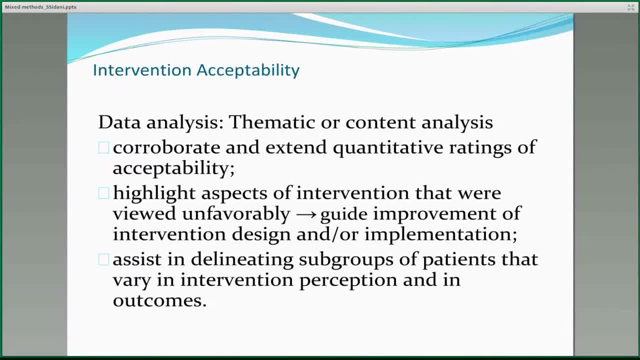 the intervention, The analysis. I use, Of course, Quantitative measures of qualitative open-ended questions usually involve thematic or content analysis and they can be used to corroborate or extend the quantitative ratings of acceptability. You know if, and usually you try to look for conversions to see of the two types of 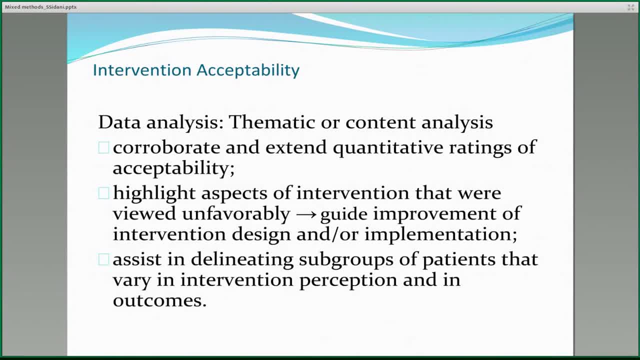 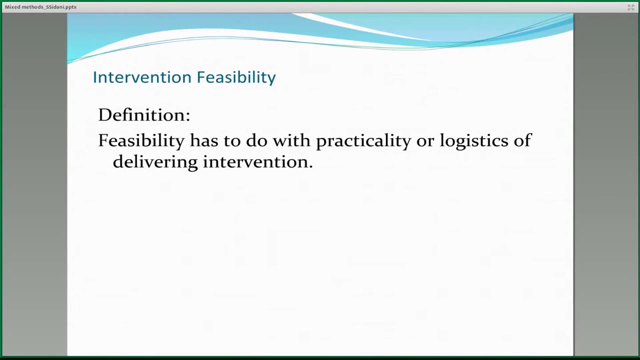 data or results to see What aspect of the intervention was viewed favorably or unfavorably and if unfavorable aspects of the intervention would need to be revised or refined in future studies. The second aspect to be evaluated in an intervention study using mixed method is the feasibility. 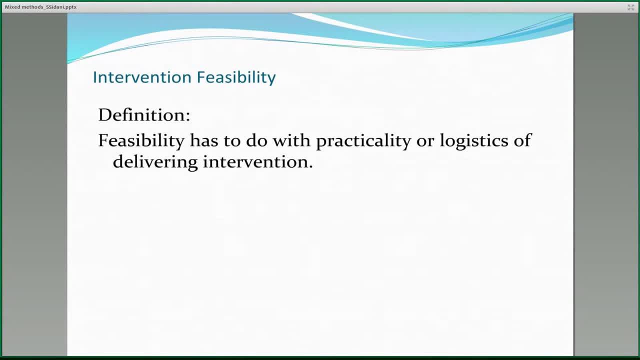 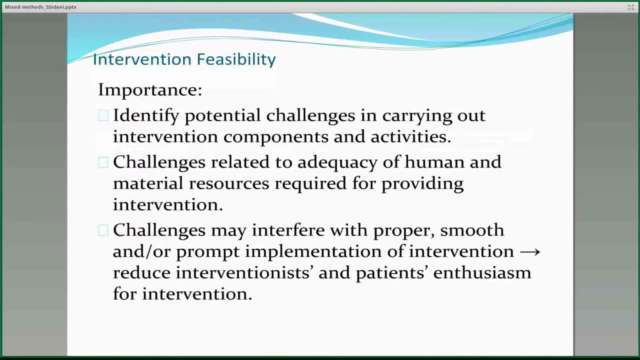 of an intervention. Okay, This has to do with the practicality or the logistics of delivering the intervention. Why do we have to examine feasibility, even in an efficacy trial? Because any challenges, any issues with the feasibility of delivering the intervention could potentially lead to, or really could potentially lead to, the feasibility of delivering. 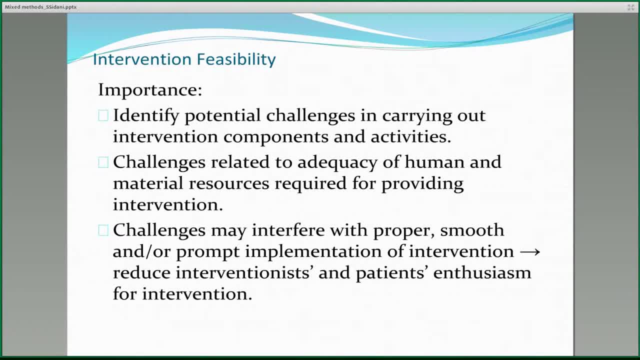 the intervention. Okay, So that's the first part, And the second part is: how do we reduce the motivation of the participant, as well as the therapist, in delivering the intervention, And if they're not quite motivated in delivering the intervention or in receiving the intervention? 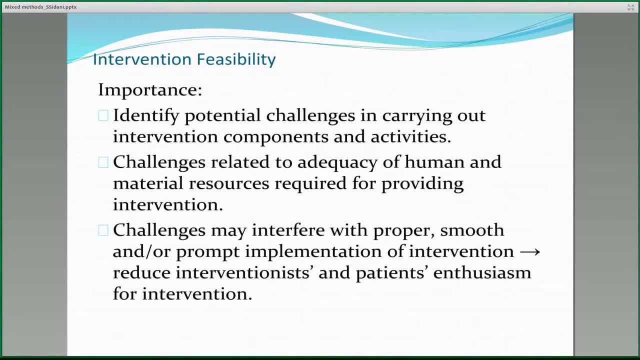 because of all these challenges, then this would lead to issues of fidelity with intervention delivery as well as the, you know, the outcome achievement. So what kind of challenges- of challenges or practical challenges- can be faced in an intervention study? Some of these challenges are related to the adequacy of the human and the material resources. 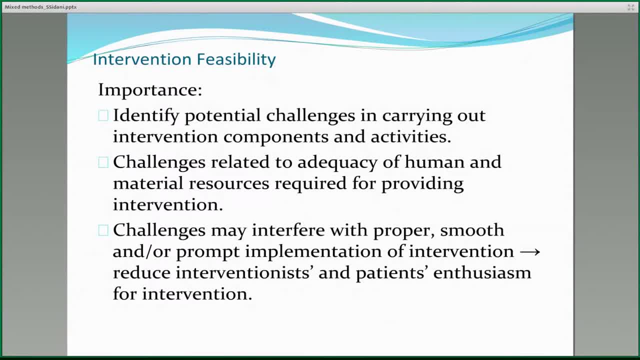 that are required for providing the intervention, And a brief example, here is an article that I was just reading evaluating an intervention that was delivered through an application, an app that people can download on their cell phone, And they reported that 80% of the participants experienced problems with the application. 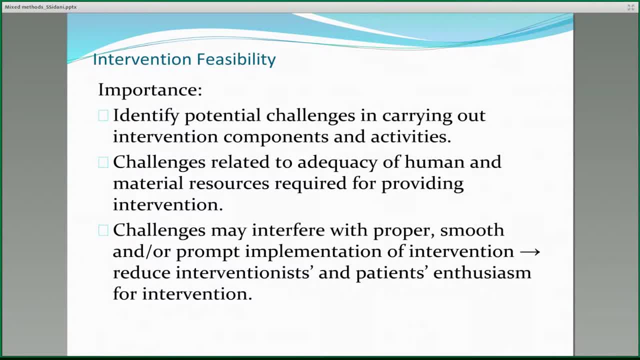 So that's an example of a challenge that in that case that I read, fortunately did not affect the enthusiasm of participants. But you know there's some challenges And some participants could be offended or may not like the fact that they have to experience. 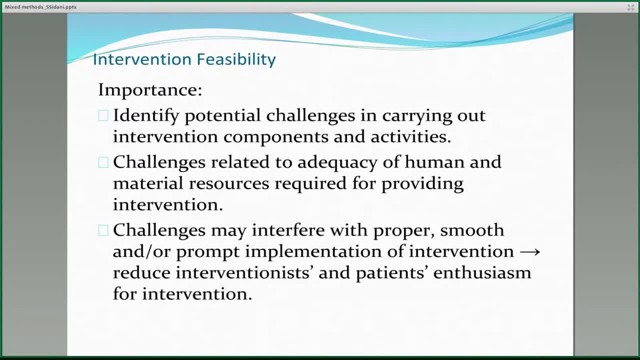 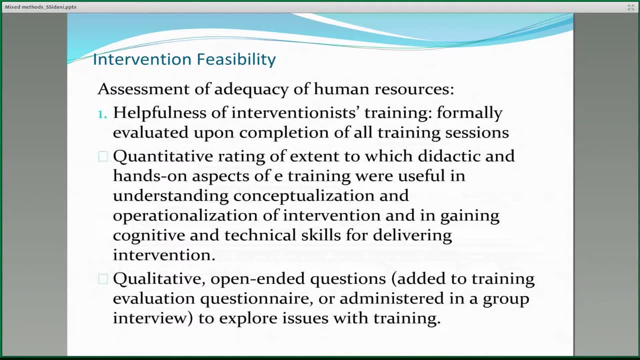 all these challenges over time. The challenges also may interfere with the proper and smooth delivery of the intervention which, as I mentioned, could affect the enthusiasm for the intervention by the interventionists and the patients. How do we assess the feedback, The feasibility or the adequacy of human resources? 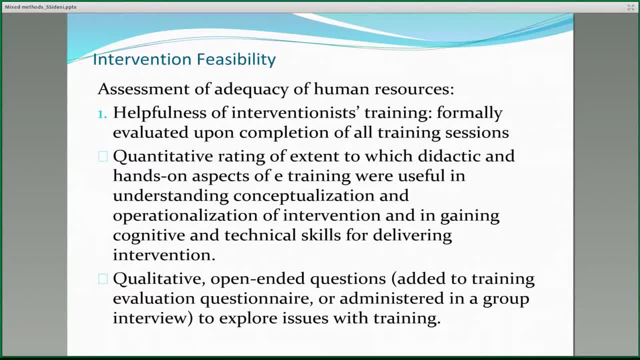 This is where we need to focus on the interventionists especially, in particular, the training of the interventionists, and determine whether or not it was helpful. So evaluating the helpfulness of the training could be done formally upon completion of all the training sessions, using quantitative rating as well as qualitative, open-ended quality. 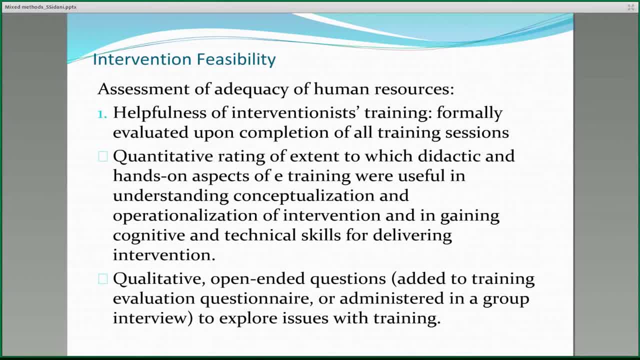 So quantitative ratings here. unfortunately, I could not find anywhere in the literature a kind of measure that has been used to evaluate the training of all or different types of interventions. So this is where the researcher will have to develop their own items for assessing the 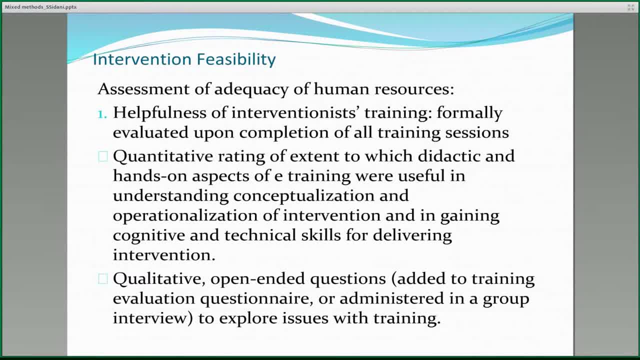 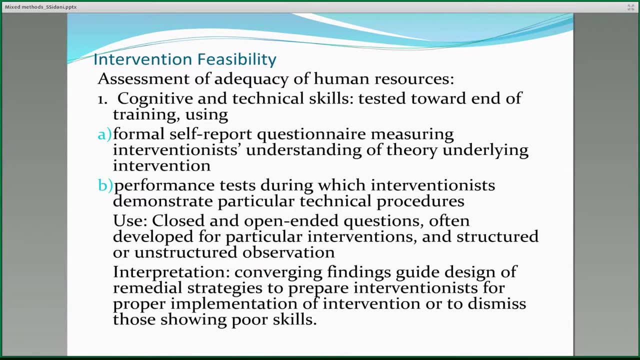 perceived helpfulness of the training. These are the open-ended questions you know to explore if there was any issues with the training. The training has to do with the cognitive and technical skills, as well as the interpersonal skills, of the interventionists. These are the different types of skills that could be evaluated in every intervention. 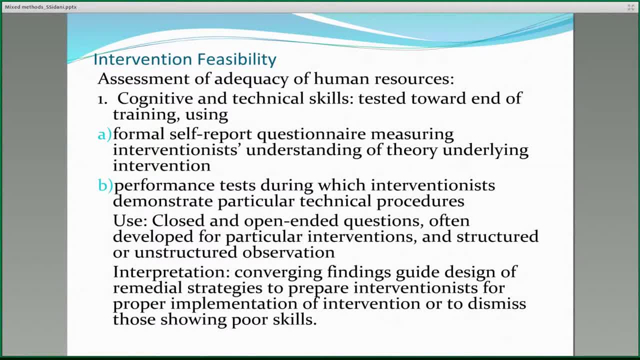 Okay study. The cognitive and technical skills could be tested toward the end of the training using formal self-report questionnaires that you, as an investigator, can develop to test whether the intervention is understood, the theory underlying the intervention. We can also design some form of performance test where you observe the interventionist. 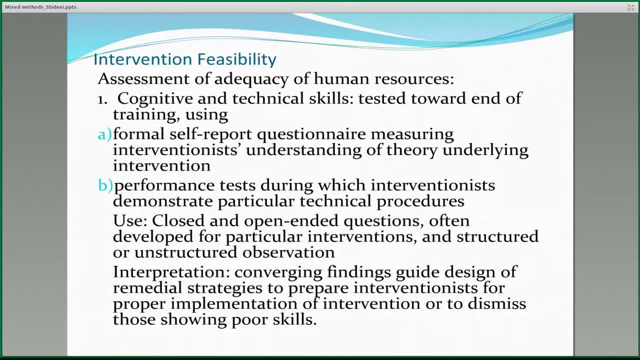 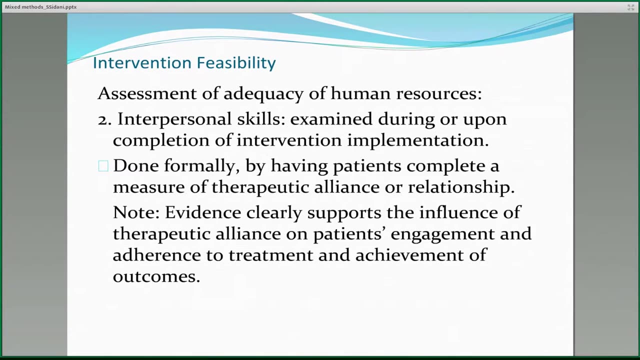 demonstrating particular skills and you evaluate them formally on that using quantitative items. The interpersonal skills Performance of the interventionist could be evaluated or examined during or upon completion of the intervention implementation, and this is usually done formally by having participants complete a measure of therapeutic alliance or therapeutic relationship. 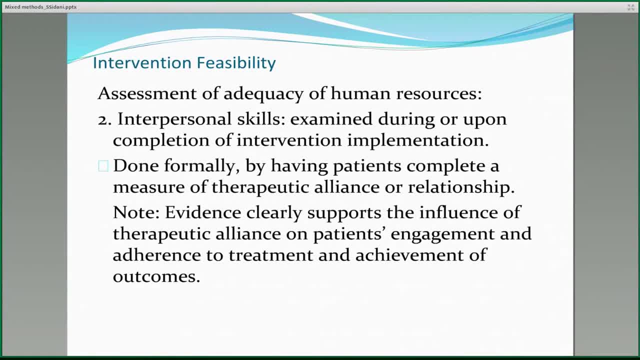 There has been quite a number of measures of therapeutic alliance that have been developed and evaluated. They have been found to be valid and found reliable and valid and could be used in different types of intervention evaluation studies. Most of these therapeutic alliance measures have been developed in the field of psychology. 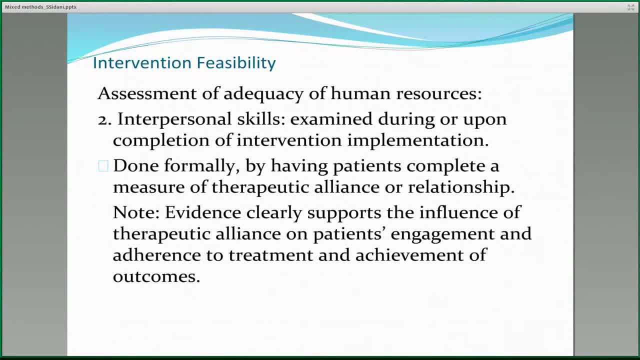 It is important for us to remember that this therapeutic alliance or the interactional style or the relationship between the therapist and the patient is important. It is important for us to remember that the therapeutic alliance or the interactional style or the relationship between the therapist and the patient is important. 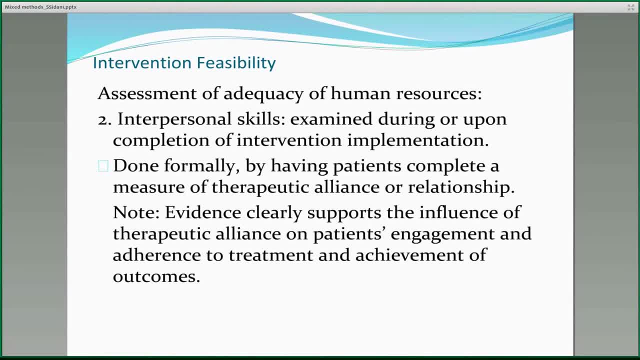 It is very important and should be assessed, in my opinion, every single intervention evaluation study, because there is enough evidence to demonstrate that it does contribute significantly to the outcome. In one of the study it made a analysis that have been done in psychology. They found out that the therapeutic alliance contributes more to outcomes than the actual. 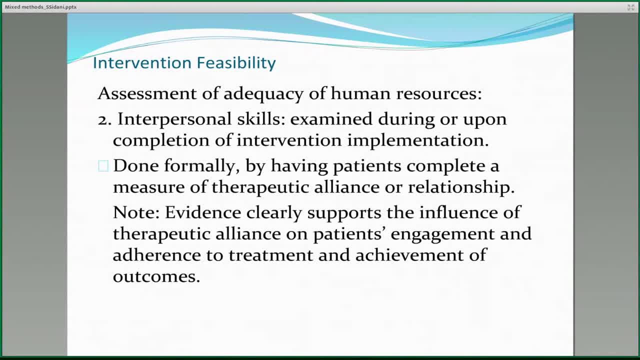 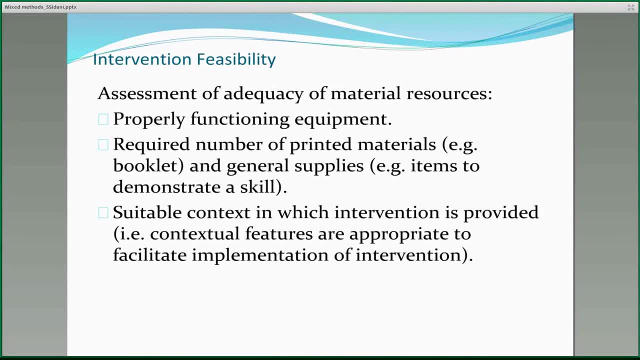 active ingredients. I think the result of that is really very interesting. Therefore, it becomes important for us to assess it, Assessing the adequacy of material resources. This has to do with the availability of everything that you would need to deliver the intervention. 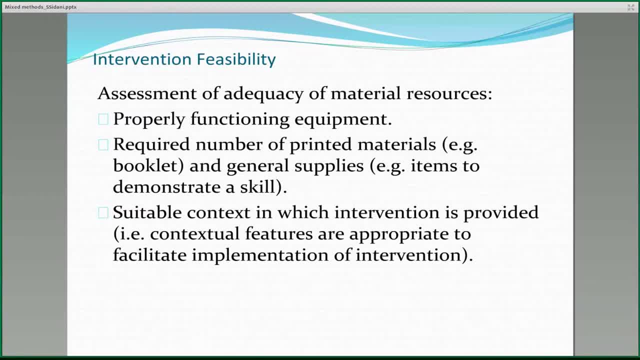 So that may include properly functioning equipment such as a laptop for computer. assisted delivery of an intervention is that you have to make sure that you have the required number of printed materials to be given to patients or general supplies that could be used within an intervention session. 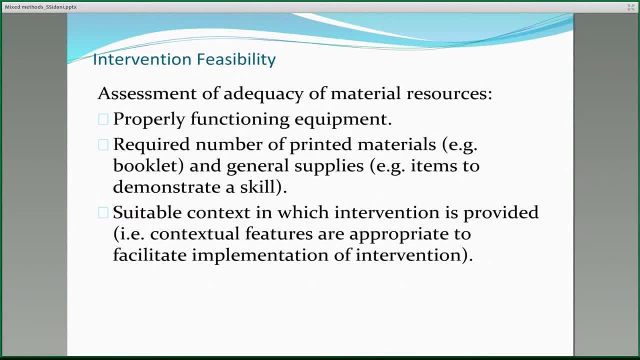 to demonstrate a skill, For instance, for those who do diabetes education, sometimes you need to have an adequate number of food items, for instance, or a menu to help them learn some of these skills, But the suitability of the context in which the intervention is to be provided should. 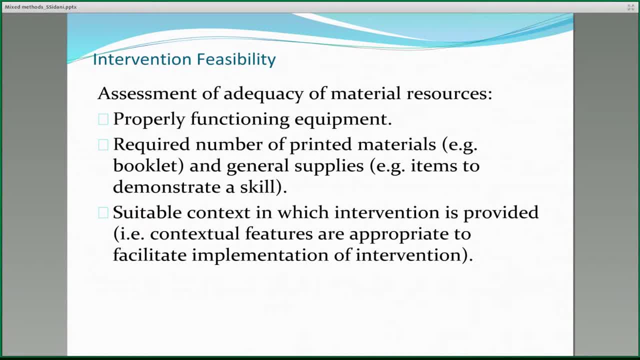 be also evaluated, because contextual features such as the location of the room in which the intervention is being delivered, the noise, collaboration among health care professionals, all of these should be appropriate to facilitate the implementation And if they're not available- all these features- then there will be potential issues with not. 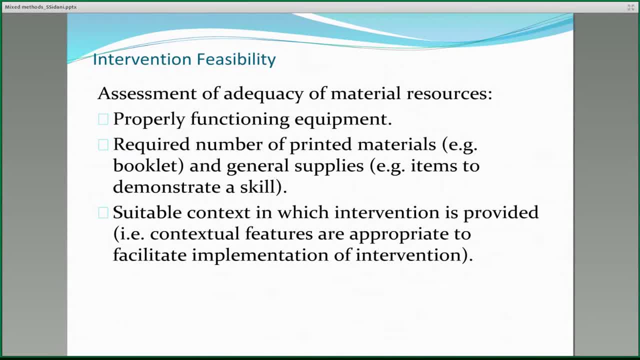 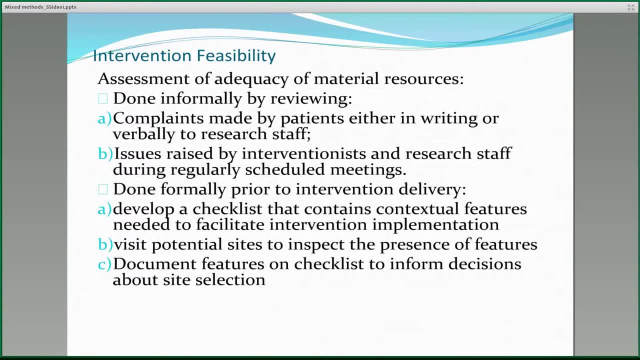 only the delivery of the intervention but, most importantly, the achievement of the outcomes. How can we assess the adequacy of these material resources? It could be usually done informally. It could be done in person. It could be done in person. It could be done in person. 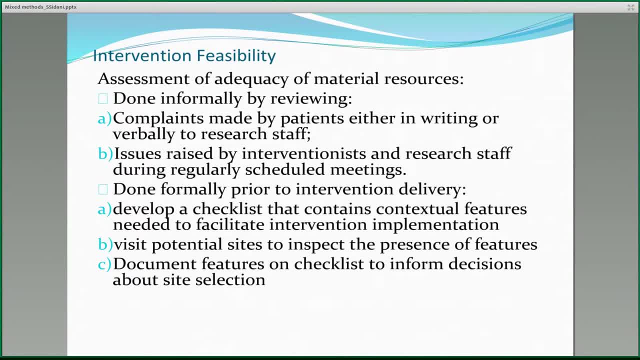 It could be done informally by reviewing complaints that were made by patients, either verbally- Some patients are very, you know, adamant and they would leave a message or email you to tell you about an issue that they may have experienced- or they may write it toward the 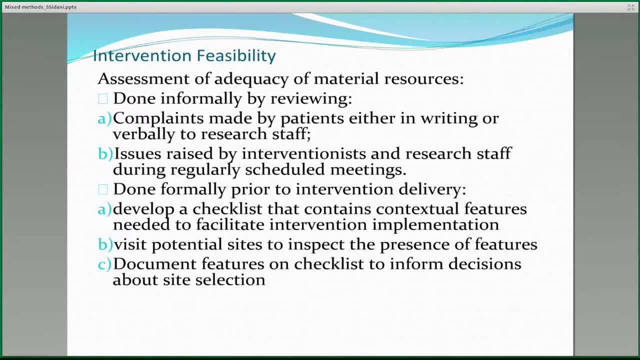 end of the post-test or whatever questionnaire that you are delivering, They may also share it with the staff. So all of these complaints should be documented per patient and then could be analyzed later. You know, assessment of feasibility, particularly adequacy of the material resources, could. 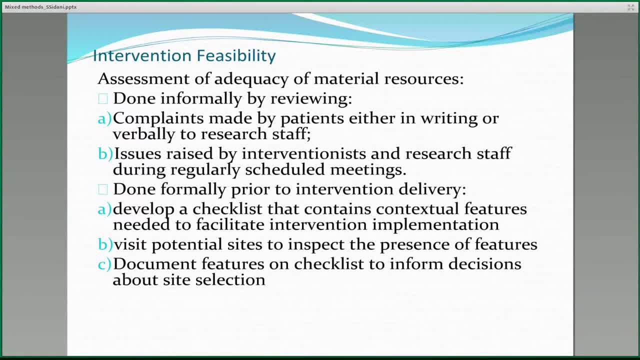 be also done by documenting any issue that was raised by the interventionist or research staff, And these issues could be, you know, raised during regularly scheduled meetings. As an example, this is an example. this is the interventionist's, interventionist's, interventionist's. 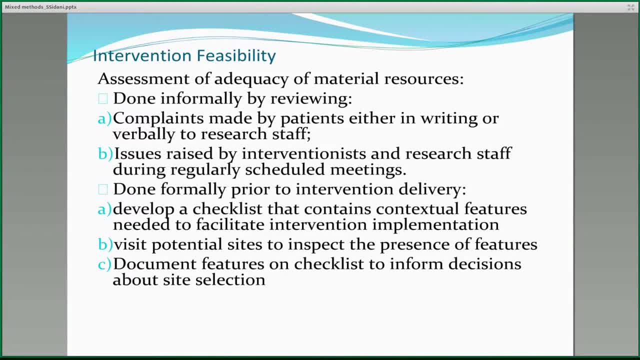 example of the importance of these contextual features is one of the studies where we thought that the intervention could be delivered in a building available on top of a subway station to make it easier for patients to come to the session during the winter time. So the site or the setting was very convenient for the participants. except that, because 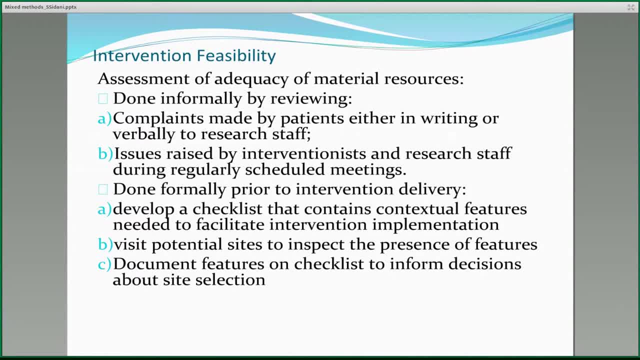 the building is on top of a subway station. every time a train passed there was a big noise and shaking that interfered with older people being able to hear the intervention. So at that point we decided to no longer continue using that setting. 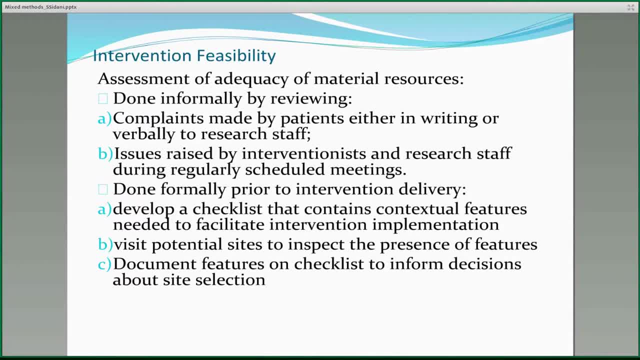 Thank you. You know the setting also could be evaluated formally prior to the intervention delivery by developing a checklist that contains all the features that you need in the particular context for delivering the intervention. Visit this potential site, inspect it for the presence of all these features. document. 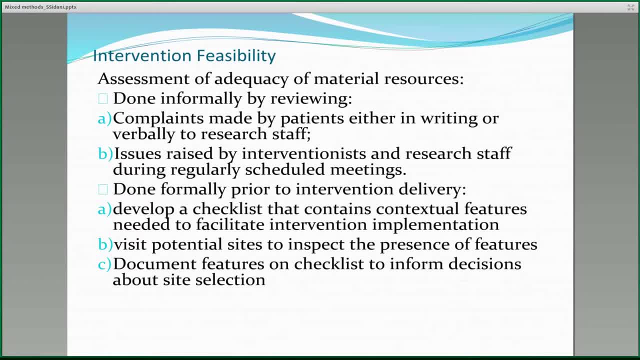 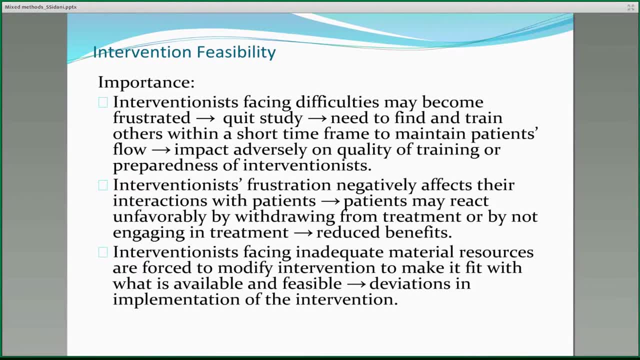 the feature on the checklist and that would help you decide whether or not to select the site for the delivery of the intervention. As I mentioned, and I briefly reiterate, the point here is that any challenges in the availability or the adequacy of the human and material resources should be documented. 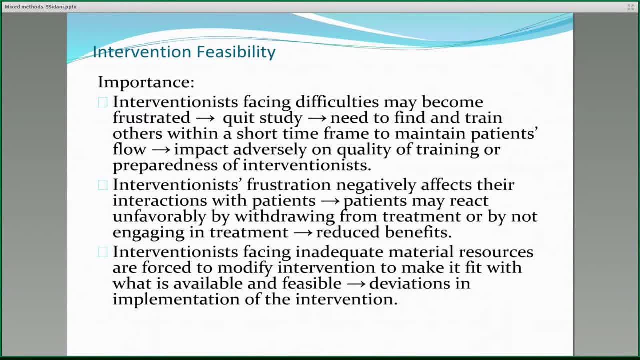 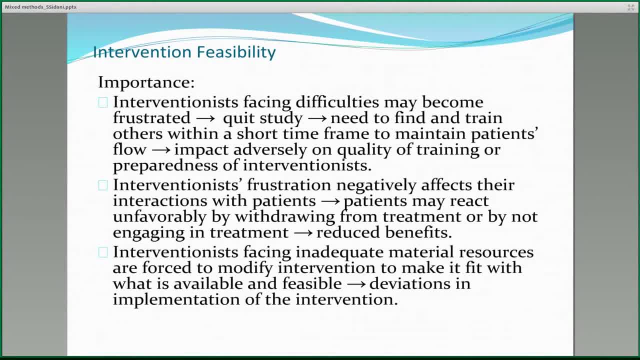 new interventionists. Some of the interventionist's frustration could be projected or it negatively affects their interaction with the patients. Patients may not like this. They may react unfavorably, which would contribute to a reduced benefit that they may experience from the intervention. 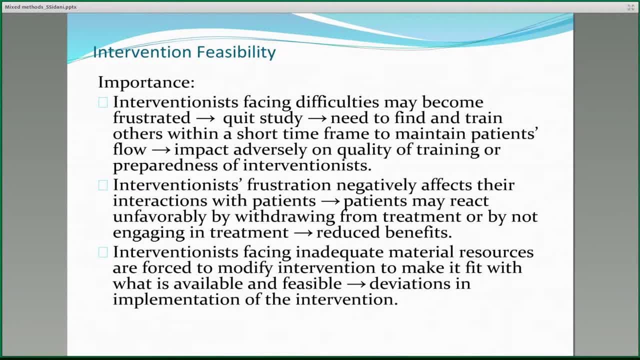 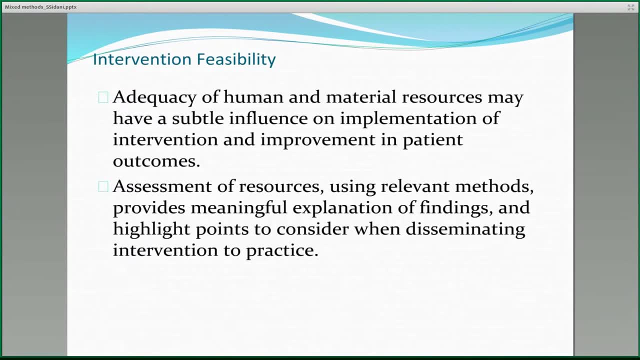 Most importantly, if interventionists face a lot of challenges in the availability of resources, they may be forced to modify the delivery of the intervention, which may lead to deviations in the implementation of the intervention and therefore, the achievement of the outcome. We have processes. 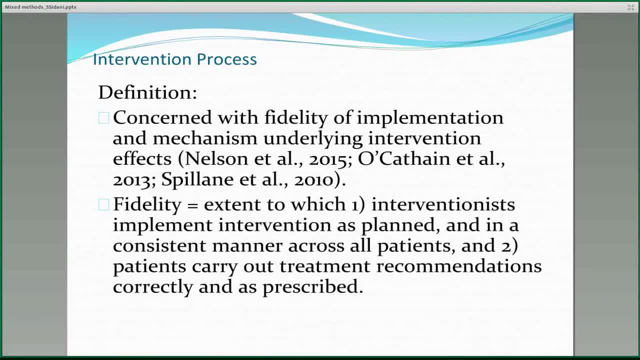 The processes also shouldof the intervention. The intervention processes should be evaluated in any intervention study, any randomized control trial, whether or not you have a qualitative or mixed methods with it, because you know it will have a lot of implications for the fidelity of intervention implementation and 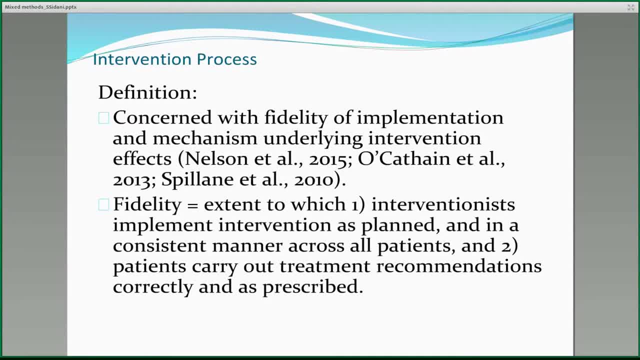 therefore the outcomes. So the process evaluation involves the evaluation of the intervention, The evaluation of the fidelity with which an intervention is implemented, as well as the mechanism that is triggered by the implementation of the intervention and is responsible for the effects of the intervention on the outcome. 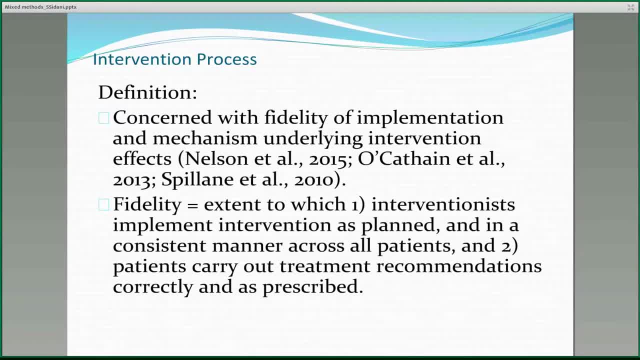 Fidelity refers to not only whether the interventionist have implemented the intervention as planned, but also whether or not the patients or the participants have implemented the intervention as planned, So the participants are carrying out the treatment and implementthe treatment recommendations correctly and as prescribed. 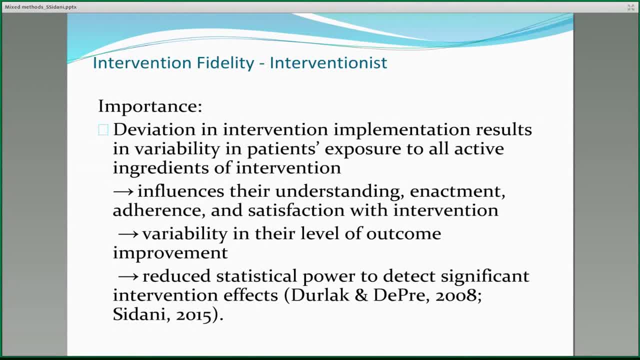 The importance of examining fidelity is that it's critical for reaching valid conclusions about the intervention effects because, as I mentioned, any variability in the implementation of the intervention on thepart of the intervention it's madeintervention is may lead to variability in the patient's exposure to the active ingredients of the intervention. 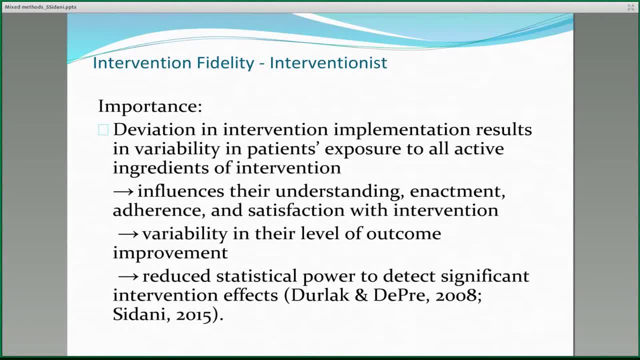 which may influence their understanding of the intervention. They may influence their enactment of the intervention, meaning that they will not apply the recommendedrecommendations correctly, They may not adhere to it and they may not be satisfied with the intervention, which would lead to variability in theirintervention. 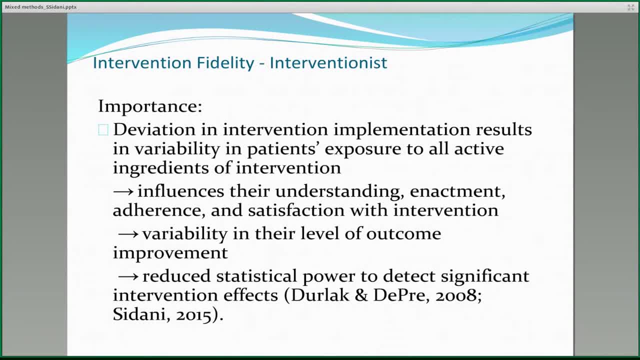 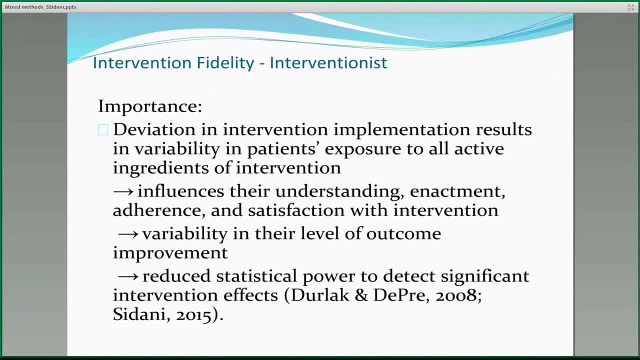 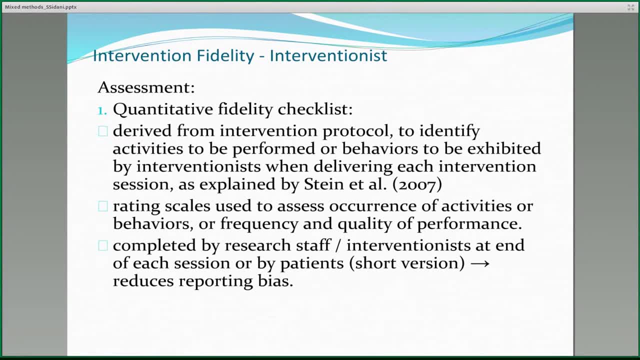 repetition. You know ease of Yes and continue to. I should I. It's beautiful. You're giving us an Lorain. Okay, that's fine. It's okay, That's fine. Now how can we assess fidelity from a quantitative perspective? 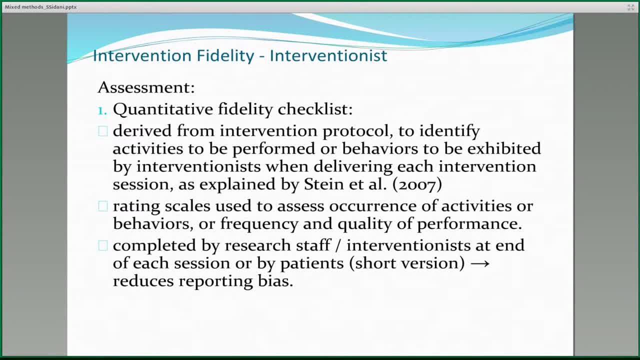 It can be done by developing a track list that contains all the items or activities or behaviors that should be performed by the interventionist when delivering every single session of the intervention. These steps have been clearly described by Stein et al in the Nursing Research article. 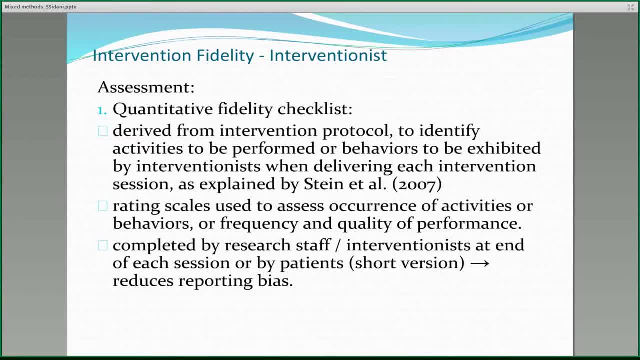 published in 2007.. For each item, you can weight whether the activity has been performed or not performed, the frequency with which it was performed or the quality of the performance. You decide on what it is that you want to evaluate the performance of these activities. 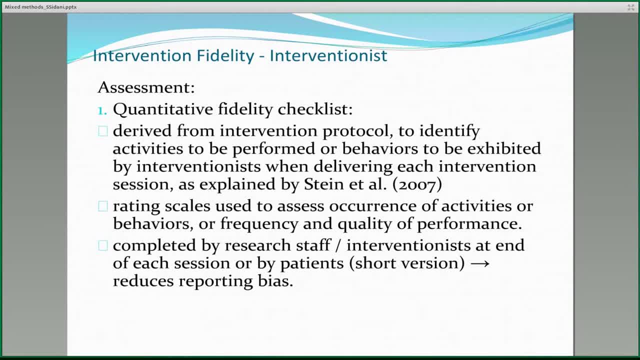 or behaviors. However, most frequently it's the occurrence of these behaviors that is reported. The checklist can be reported by the research staff or the interventionists themselves. I can suggest also that we can have a shorter version of this checklist that could be completed. 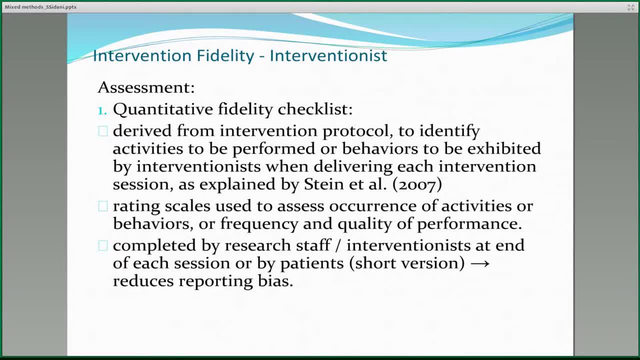 by a patient to help us understand the patient's perspective. I can suggest also that we can have a shorter version of this checklist that could be completed by a patient to help us understand the patient's perspective or perception of the extent to which the intervention was delivered as planned. 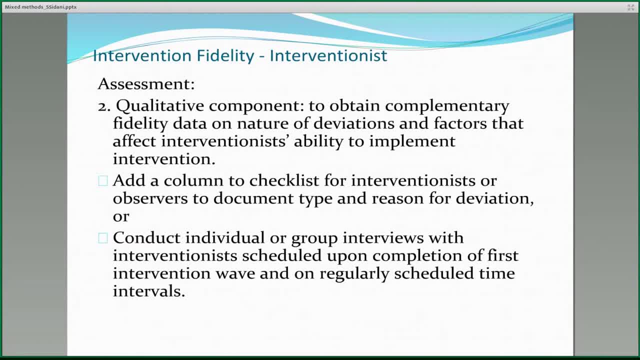 Qualitatively, the fidelity can be assessed using different formats. here, One of these qualitative ways of collecting data on fidelity is to have unstructured or non-structured data, To have a structure that is more or less consistent with the data that you're collecting you. 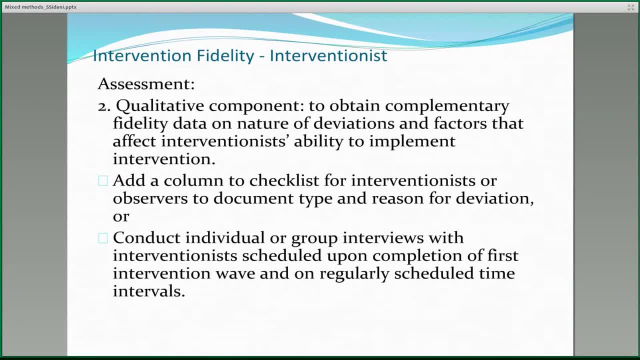 can use the data that you're collecting. So if you have a data that's not consistent with the data that you're collecting, then you can use the coupon code for permission to do a little re-to-do In our tool kit. you'll find very helpful notes, let's say, about how to control behavior. hornig listed in picture because again, this topic is rather important. But we do want to sell this, this data, evenly so that the patient doesn't be going into trouble and shop the data. there's a whole bunch more right now that has different Interestingly. 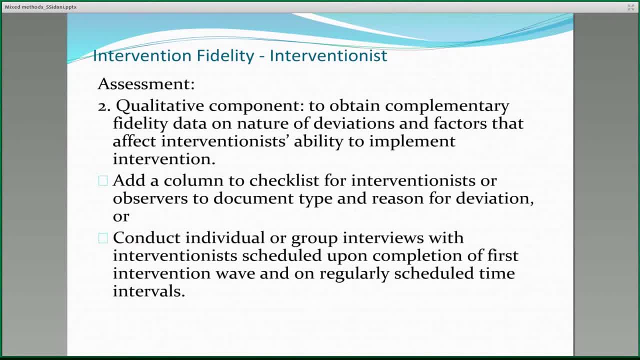 the load-up number on, for instance, the function of the control tower of the tweet, And it's important you need to have both protection history or of the testing to be insured. This also helps you to use— to recognize if the consistency is absolutely consistent. 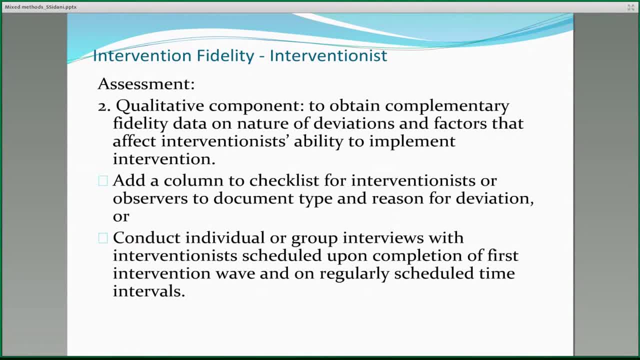 vendor information or something that you need for the end user to charts all of the data that they might need In the manuals. Of course, that asks the question: can you describe what that looks like? that data? you can add a column to the checklist where the interventionist or the observer 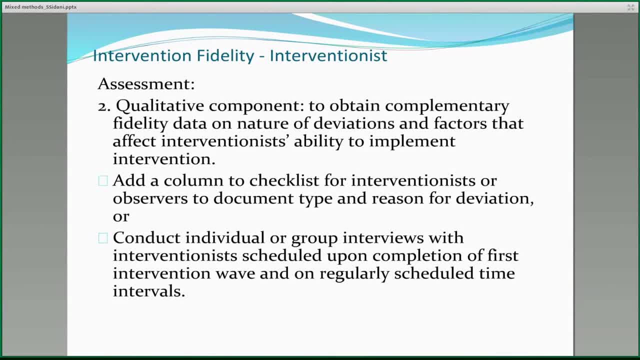 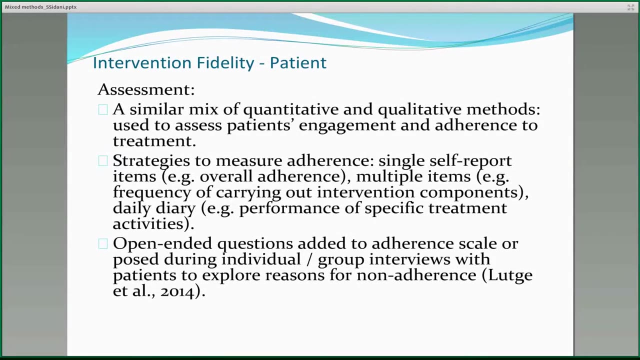 can document this information or you can plan on having an individual or group interview with the interventionist to ask them about. you know, how did they implement the intervention, what were barriers and facilitators, What kind of quantitative and qualitative methods or strategies could be used to assess. 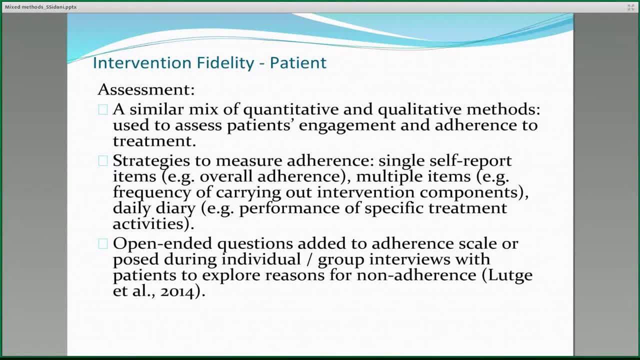 adherence of the patients to the treatment. There are plenty of quantitative measures that are available in the literature and you can add open-ended questions at the end of the adherence scale, or you can hold interviews with the participants to explore reasons for non-adherence or not only the reasons for 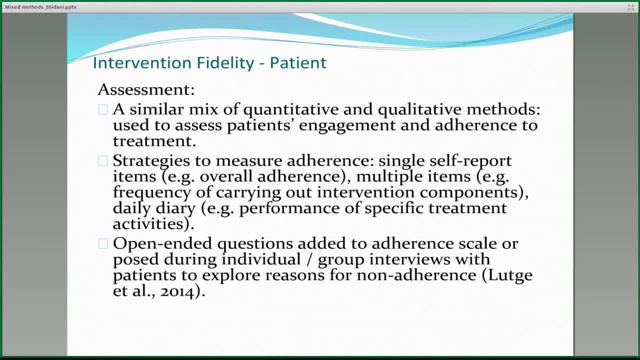 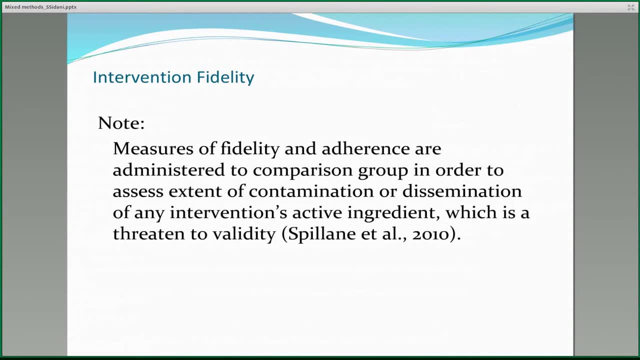 non-adherence. But you know what are the reasons for non-adherence, What are other factors that may have, you know, led them or contributed or helped them in applying the intervention recommendations. It is important also to assess the fidelity and or fidelity of the intervention delivered. 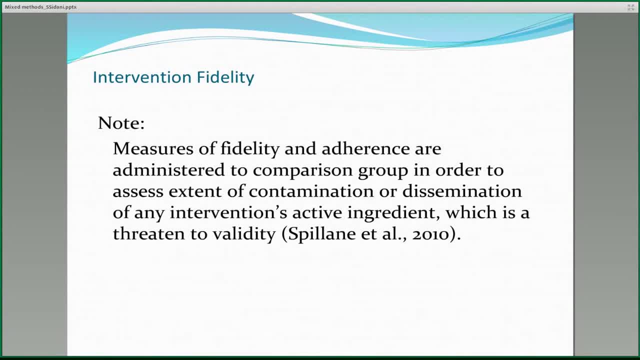 by the interventionist or adherence of patients to the intervention in the comparison group. This becomes important to determine whether or not there has been contamination or dissemination of any aspect of the intervention's active ingredient. This is important because if you have a contamination of the intervention that that could potentially 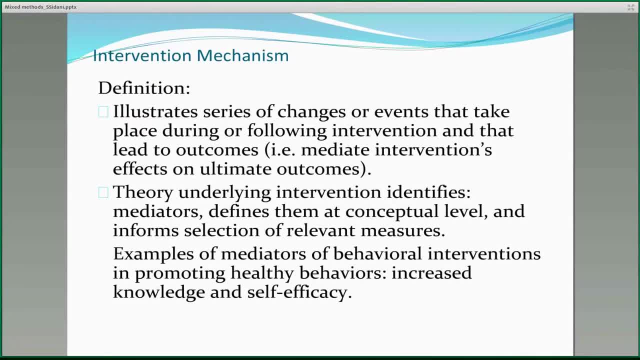 explain non-significant findings in terms of the outcomes. Evaluating the mechanism of the intervention effect underlying the intervention, In fact, on the outcome is important because the mechanism is a series of changes or events that take place after delivery of the intervention that could contribute to the achievement of. 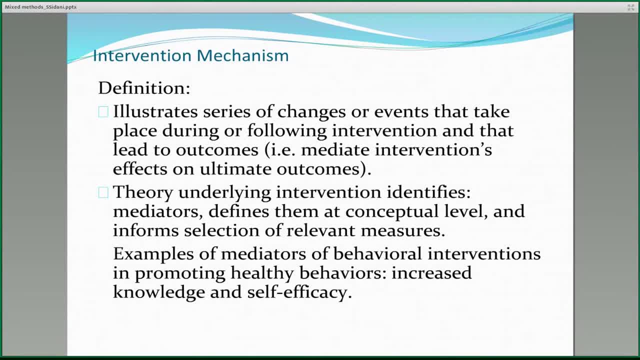 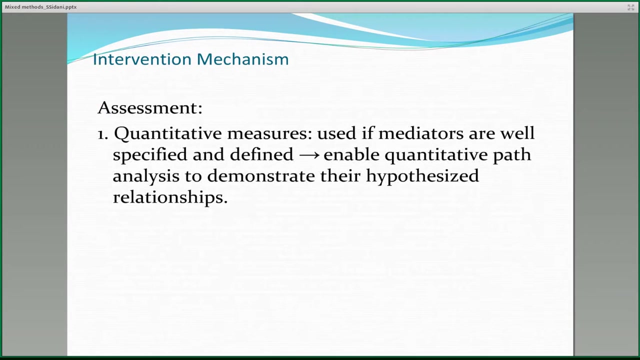 the outcome. Where do we get these mechanisms? Usually, the mechanisms is usually specified by the theory underlying the intervention. The theory, would you know, determine or tells you or informs you about possible mediators of the intervention effect on the outcomes. Examples of mediators for behavioral interventions are increased knowledge and self-efficacy. 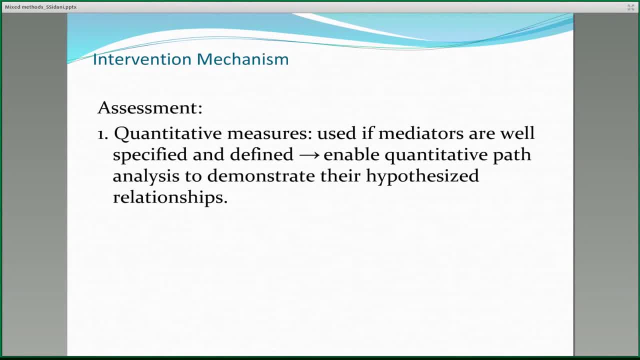 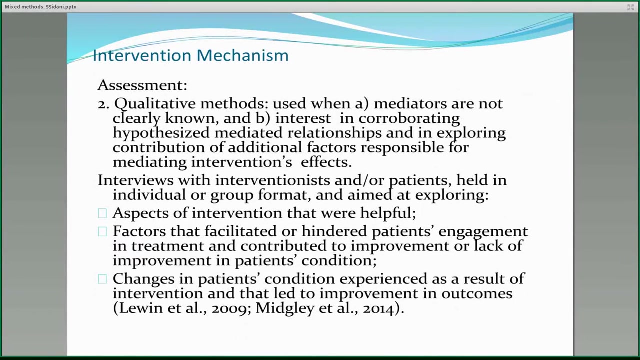 Quantitative measures can be used if you know what are the mediators. based on a theory, You have a theoretical, conceptual definition As well as operational definition. that would help you or guide the selection of available measures to assess the mediators When these mediators are not well known or a priori, or if you are interested in corroborating. 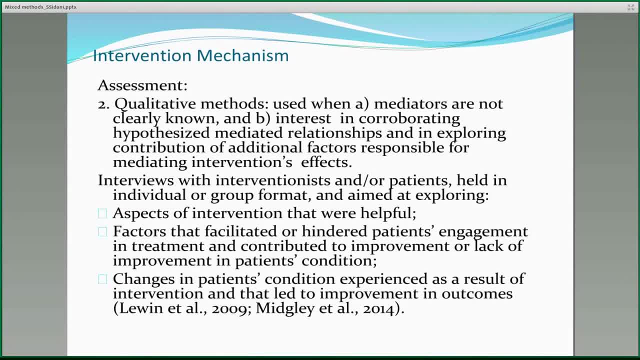 the hypothesized mediators. you can add qualitative methods by interviewing interventionists as well as patients And ask them about aspects of the intervention that were or were not helpful, factors that facilitated or hindered the implementation, or patient's engagement in the treatment, or 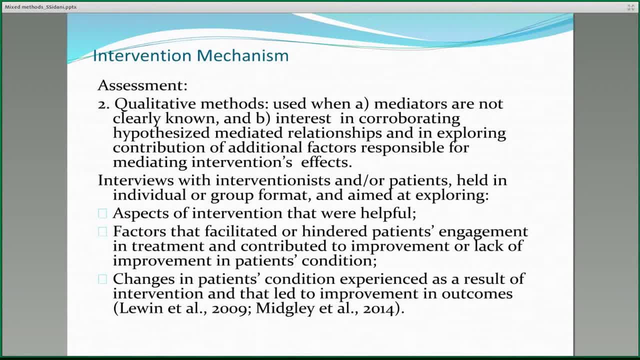 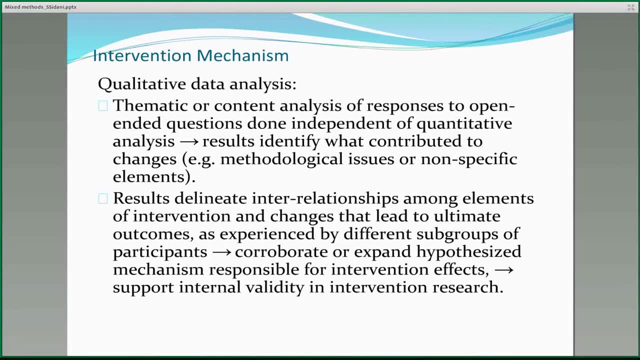 the intervention and contributed to the outcomes or lack improvement in their outcomes Or any other additional changes that the patients may have experienced as a result of the intervention. You know these are the main things that you need to know. Next slide: These qualitative data could be analyzed thematically or using content analysis and. 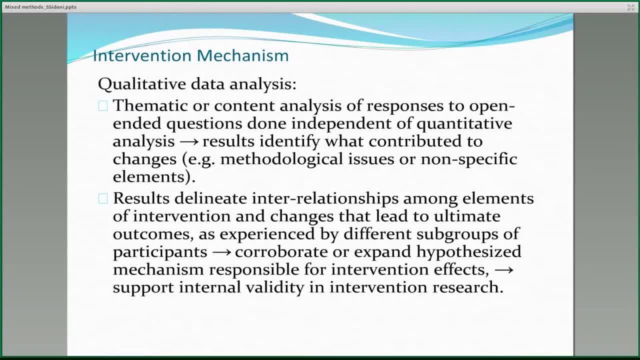 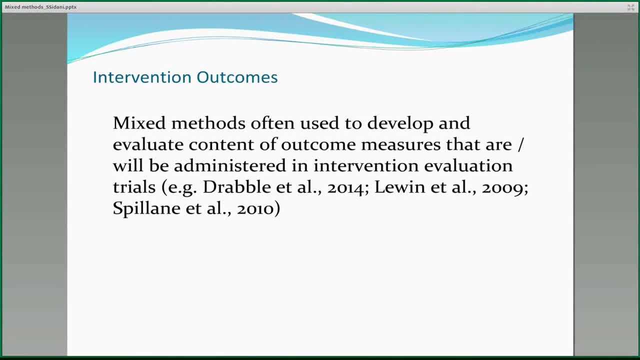 they will help you to determine what contributed to the outcomes, Because it becomes important. I was just reading an article where the researchers conducted a similar kind of interview toward the end of the study to ask them in their perspective, using qualitative methods, What contributed to their improvement, especially that the quantitative data analysis have demonstrated. 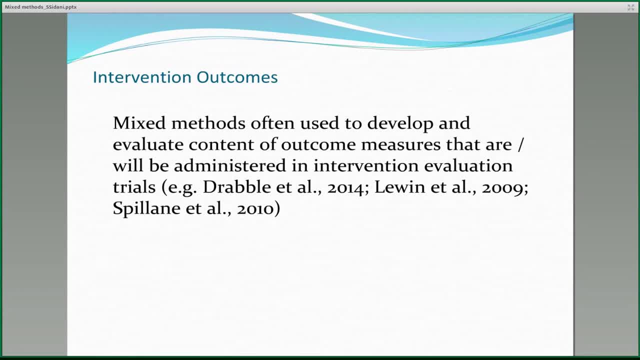 that people or participants in the comparison group have demonstrated improvement, And by conducting these qualitative interviews with participants in both the experimental and the comparison group, they found out that asking the patients to monitor their symptoms made the difference. They led people in the comparison group to act on their symptoms and therefore explained. 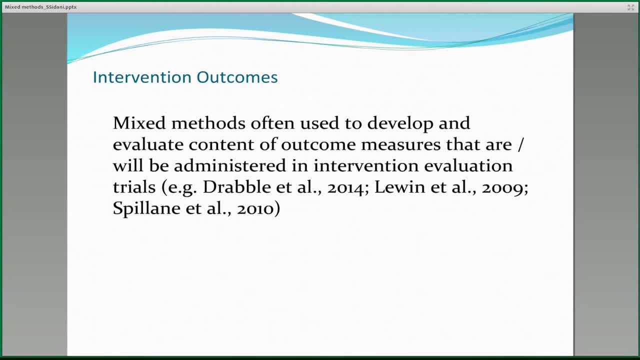 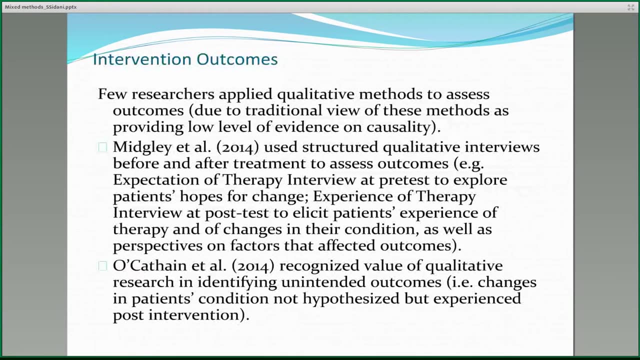 why they demonstrated the improvement. Using mixed method is also now being recommended to not only develop and evaluate the content of outcome measures that will be used in a trial, But also to identify possible outcomes. So this is a good example. Next slide: 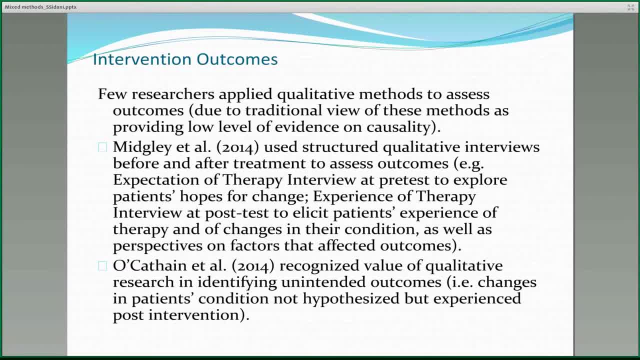 This is a slide where we have two authors that have given more information on how you can use structured or middle, middle, middle, ah, I cannot pronounce the name of the first author listed. They suggested structured qualitative interviews that can be used to assess the participant's expectation of improvement at pre-test, as well as the experience. 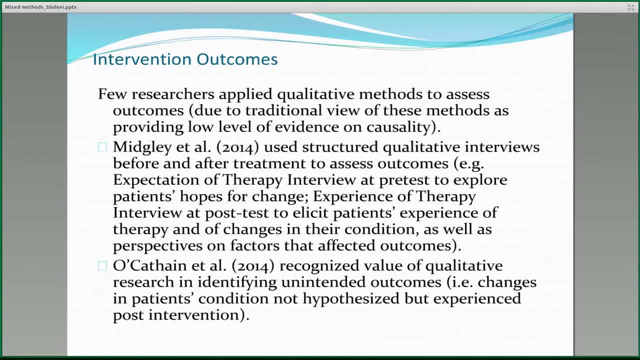 with the therapy at post-test OCAFENES, and colleagues have recognized the value of qualitative research in identifying unintended outcomes, meaning these are changes that would occur in the patient's or the participant's condition that has not been hypothesized a priori but has been experienced. 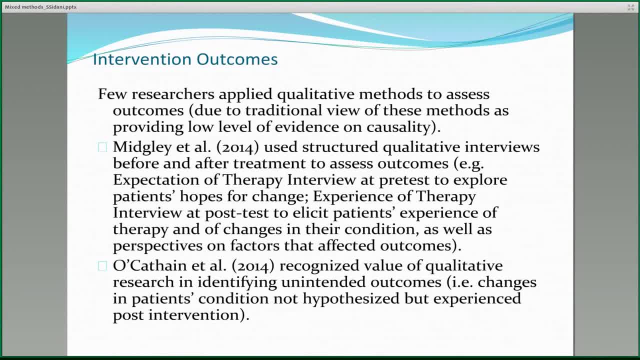 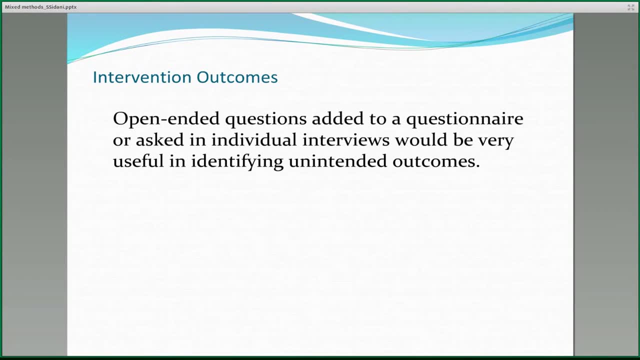 And this is very important because it does help you identify potentially positive or favorable benefits to your intervention that you may not be aware of. How can you do that? You can do it through interviews, or the way we have used it in our previous work is to 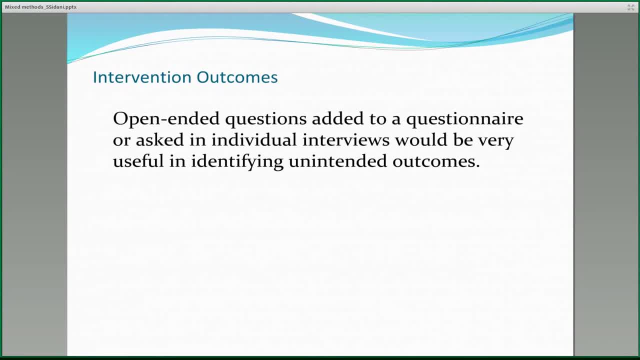 add one open-ended questions at the end of a post-test questionnaire asking them: how did your intervention affect you in a positive way and how did it affect you in a negative way? You will not get an answer from every single participant, but some would write very short. 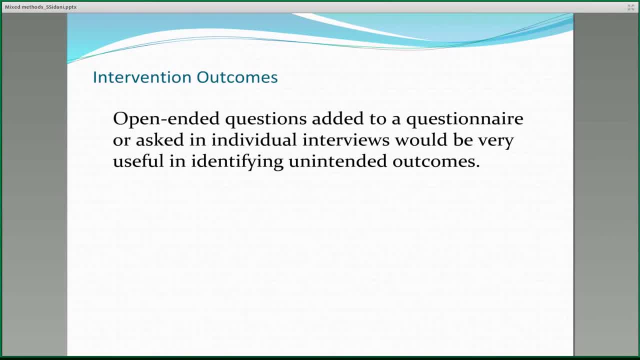 answers that are as informative as really long answers, But it's better than nothing. If you can afford, you know, from a research point of view it's better than nothing. And if you want to be as broad-minded from a resource perspective and time-wise to hold, 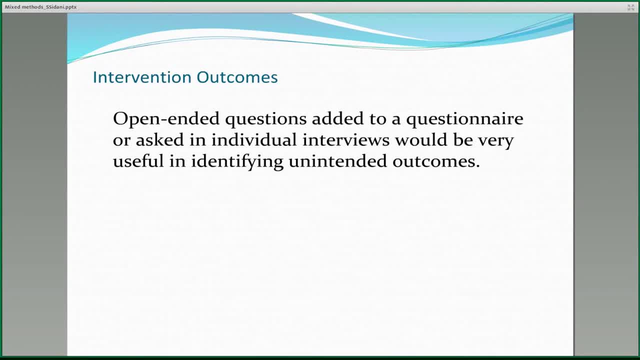 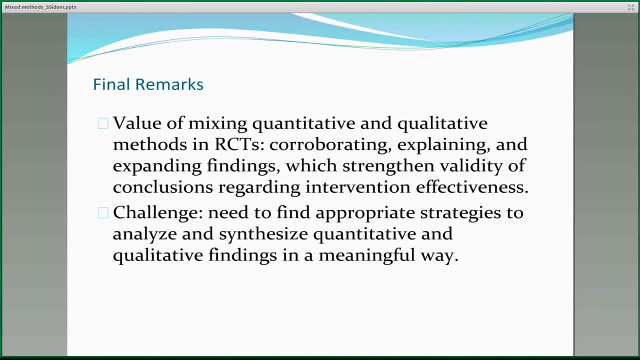 interviews with individuals. that would be great. I will conclude, because I'm over time probably, with reiterating the importance of mixing quantitative and qualitative methods in an RCT, because they will strengthen, especially if the results corroborate each other or, you know, converge. they would strengthen the 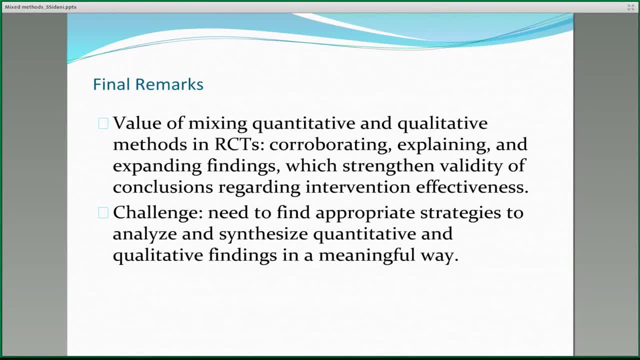 a validity of the conclusions. If there is diversions, it would get you to think more, or try to think about what is going on, And I think I'll stop here. Thank you very, very much, Soraya. That was a very interesting and a wealth of information. 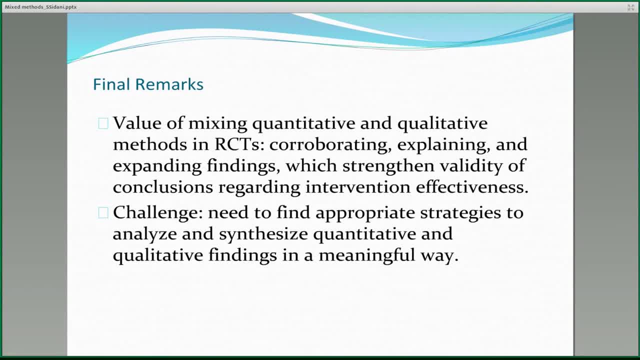 I think we have time for a couple of questions. Does anybody have a question? You can put it in the chat And I'll just read it. Or if you have a microphone and want to put up your hand As I'm just waiting, sorry, go ahead. 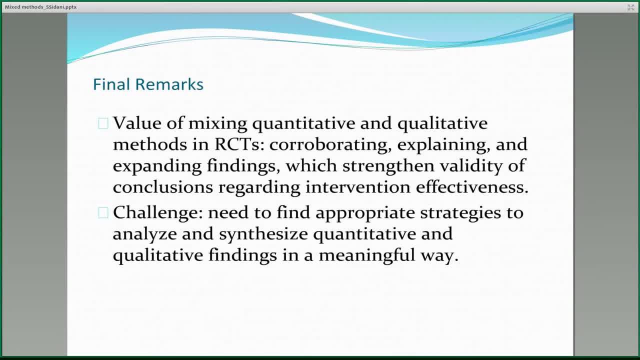 Someone have a question? Sorry, I couldn't quite catch that. Do you want to just write it in the chat? Soraya, I just wondered if you could talk a bit more about the comparison group and how you would see the best way to use the qualitative inquiry. 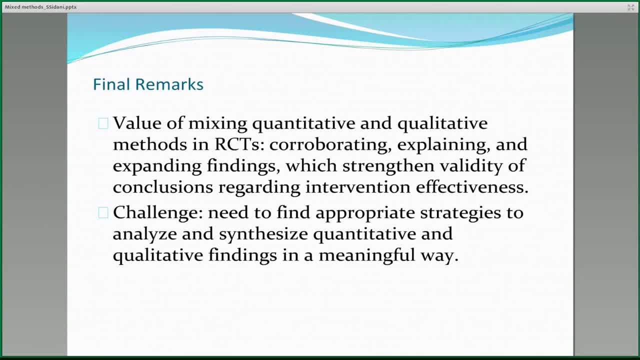 Okay, It depends on your intervention and what it is. what is the intervention and what are the components, the active ingredients of the intervention, as well as the nonspecific elements, Because a lot of the comparison conditions may involve, or particularly those that have been designed around structures plus table. you may deliver the nonspecific elements. 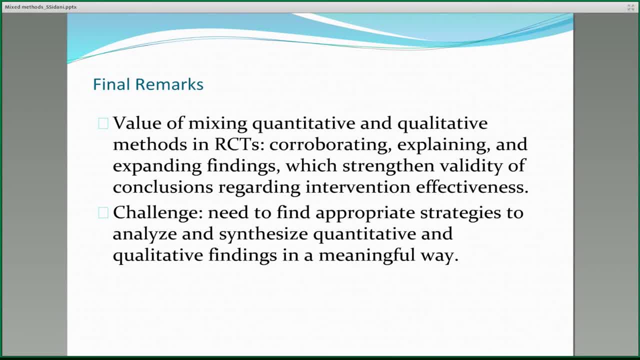 To them to make the placebo, for instance, comparable, or the comparison treatment comparable to your intervention delivery. but these nonspecific elements could potentially lead to improvement in the outcomes, So I would. it would be interesting or important then to interview for intervention. 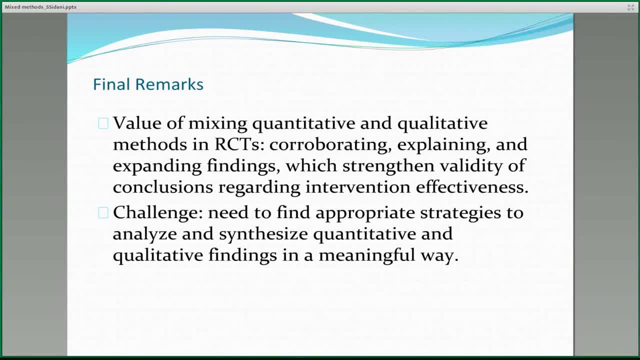 I think that's a good point. I think that's a good point, Thank you. Thank you, And that's great. It's a good point, Thank you, And I would also like to ask if you had been involved in any of the interventions that. 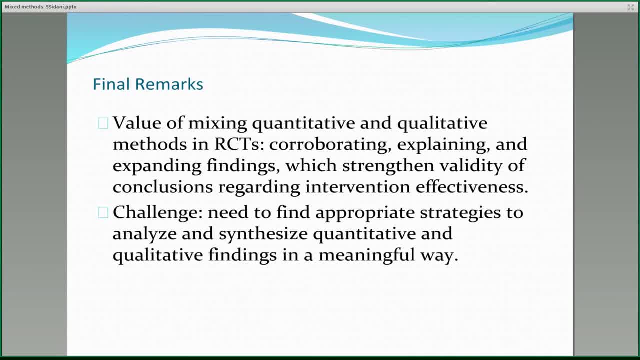 have been conducted or what you consider to be the most significant and the largest intervention that you've had, that you've had in your model. I see, thank you OK, And I would like to ask: is there, is there a challenge to the patient setting? 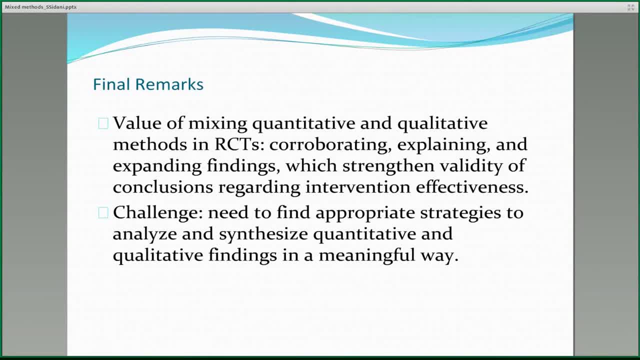 up for these interventions? to each individual intervention: Yes, We have some of the interventions that we have done and we've had some of the interventions that women have had, for instance, or asked these open-ended questions about what they thought about the intervention or the treatment group or the group to which they have been. 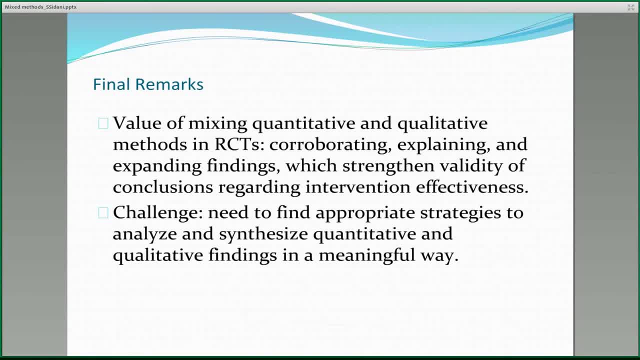 assigned? did it affect them in any way, and how did it affect? Did I answer your question, Wendy? Yes, that's very helpful. Diana's got a question. She said I noticed that Dr Sedani mentioned open-ended questions. 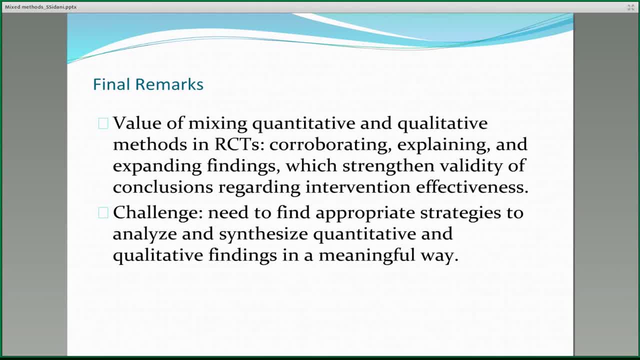 Does she have experience with observations or mystery clients to collect qualitative data? Personally, I have not used unstructured observational qualitative methods in my own research, But where this has been used a lot is in program evaluation, especially evaluating complex programs delivered in the real world. 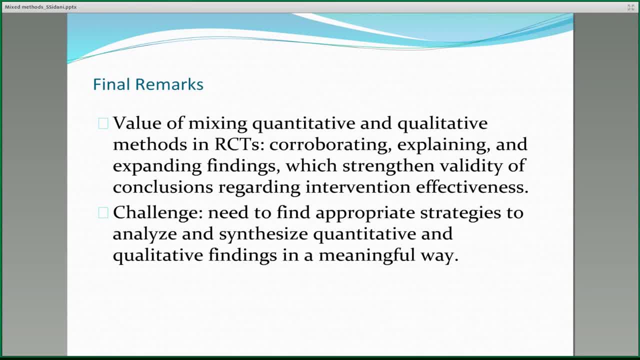 You want to know how therapists, interventionists or health care providers are implementing the program, And if the program is too complex or you're not quite sure exactly what the program is all about, as may be the case sometimes in a lot of these publicly funded 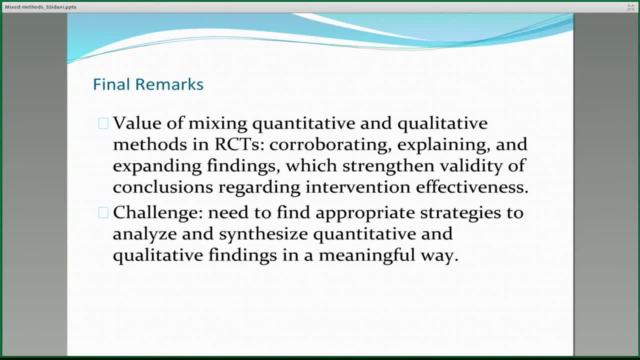 programs. you can send your research staff to do observation and see. So that would be something like what has been done in the work to evaluate the research. Thank you, Is there anything else that you would like to add? Yes, So in the program the program is. 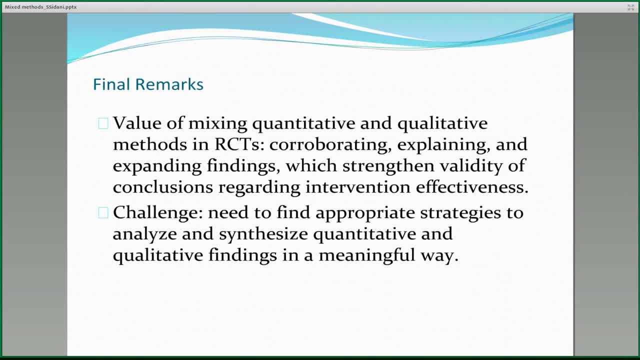 designed to evaluate the nurse's work. I forgot what they call it, something in motion, where they would observe every single activity or behavior performed by the person delivering the treatment. So I will refer Diana- or I think it was Diana- to program evaluation literature about using unstructured